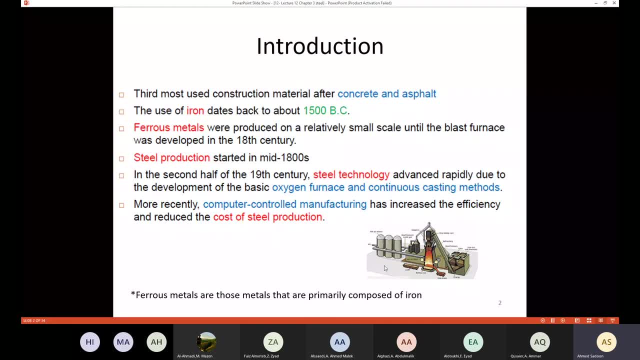 the invention of the blast furnace. So here is a blast furnace just like a big furnace with a special equipment. So after the invention of the blast furnace the production of the steel has been produced on large scale. So steel production started in the mid 1800s. 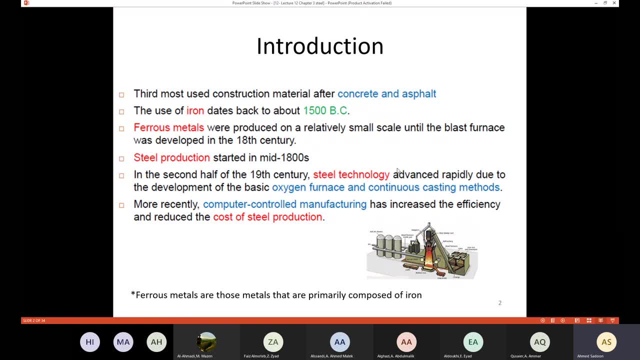 In the second half of the 19th century, steel technology advanced rapidly due to the development of the basic oxygen furnace. So, again after the invention of the blast furnace, we have another type of furnace: oxygen furnace. This furnace is used to reduce the amount of carbon in the steel and also in order to 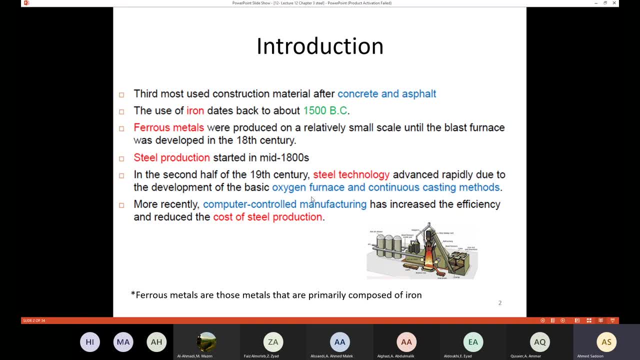 remove the impurities. So also this one helped the production of the concrete. And also we have the continuous casting method, which means that after we got the steel directly, we are going to produce the materials from the steel And nowadays, more recently, we are producing the steel from the steel. Now, this steel. 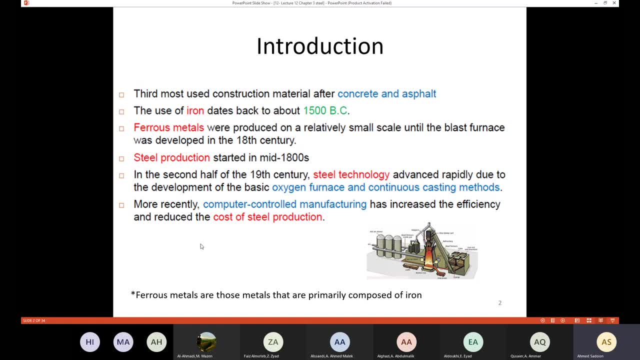 computer-controlled manufacturing has increased the efficiency and reduced the cost of the steel production. So, in order to sum up all of this, we know the steel from a very old age, but with the invention of the blast furnace, that increased the scale on which we produce steel, then the 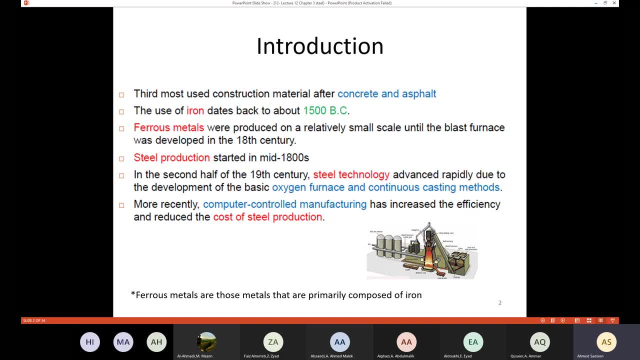 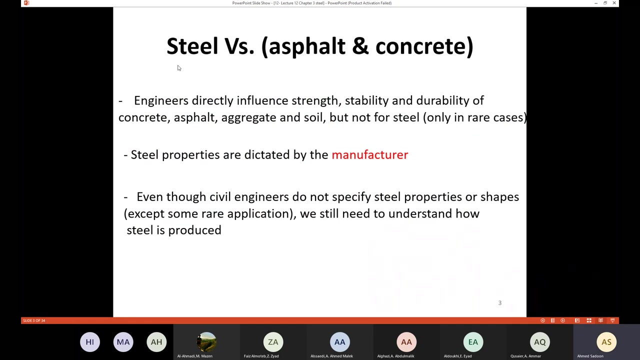 process became quicker with the oxygen furnace and the continuous casting method And nowadays we are using computers which increase the efficiency of the production of the iron. So we need to compare the small comparison between the steel and the asphalt and concrete. So, as in the case of the steel, we have a small comparison between the steel and the asphalt. 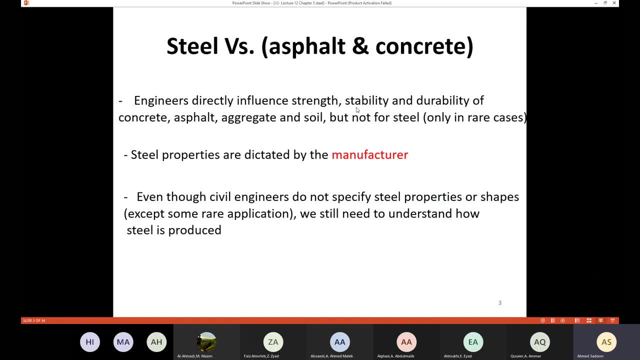 So, as in the case of the steel, we have a small comparison between the steel and the asphalt. We directly influence the strength, stability and durability of the concrete, asphalt aggregate and soil Right. So as engineers, we can influence the strength and the stability. 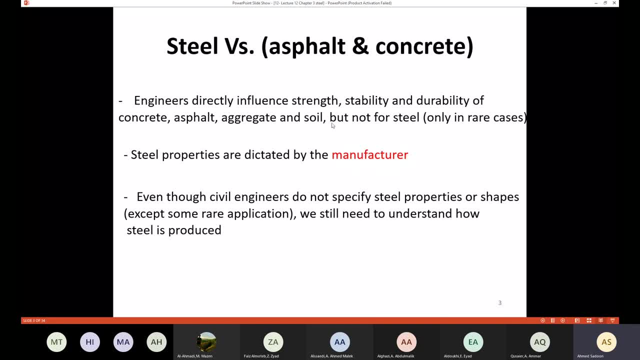 and durability, like we have studied about the asphalt and the concrete, But we cannot do that for the steel. Of course, only in rare cases, But generally speaking, we will not be able to directly influence the strength, stability and durability of the steel. 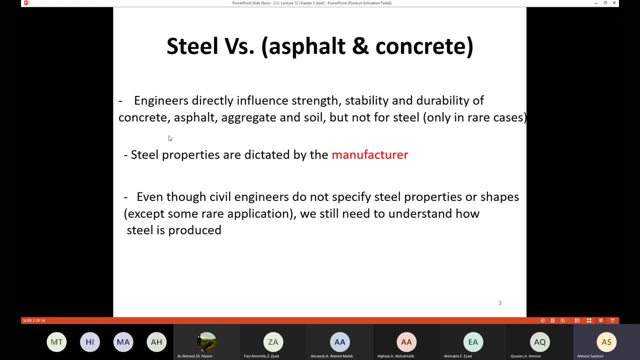 So who is going to control all of this? Steel properties are dictated by the manufacturer, So the manufacturer is going to set the terms, not you as an engineer. So even though, as civil engineers, we do not specify steel properties or shapes, of course, except in rare application, 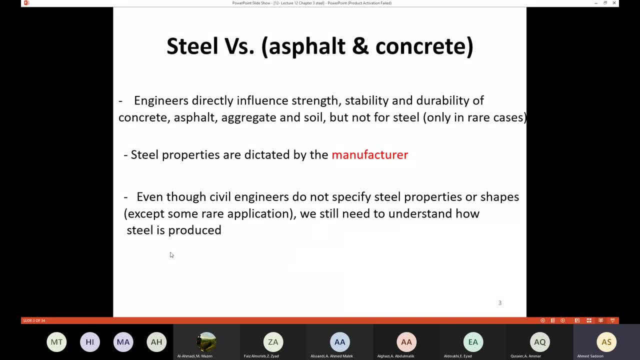 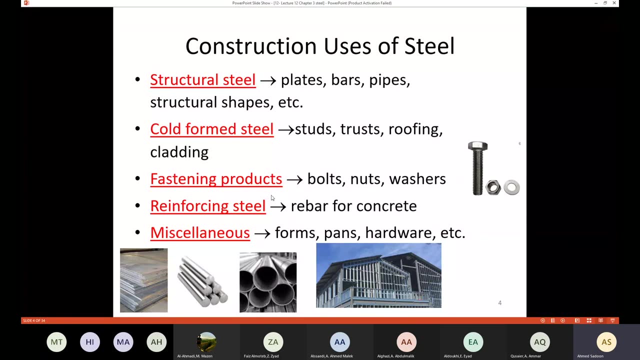 we still need to understand how steel is produced, Even though we are not going to set the terms in order to produce the steel. but it's important for us to understand how the steel is produced. So we have different types of steel in construction. 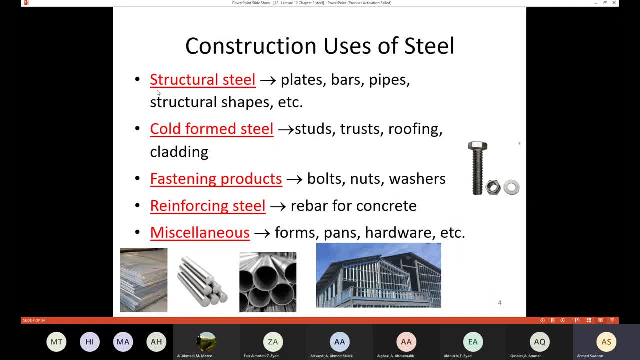 We use different types of steel. We have structural steels like the blades. The blades- this is the blade here. It could be used. It could be used for floors and so on. We have the bars, like this one. We have the pipes. 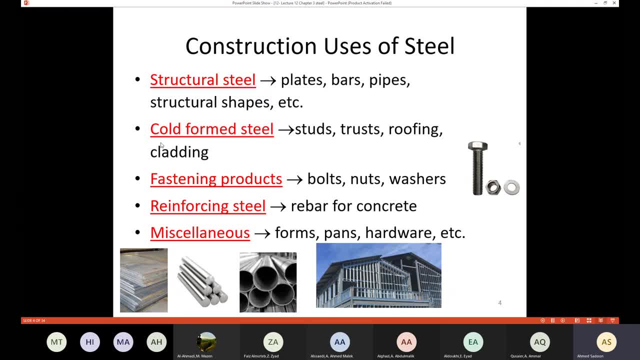 And we have many structural shapes. Also, we have the cold-formed steel, like the studs- this one here, Cold-formed studs, like the trusses and like the roofing and the cladding. Also, we have fastening. We have the fastening products like the bolts, nuts and the washers. 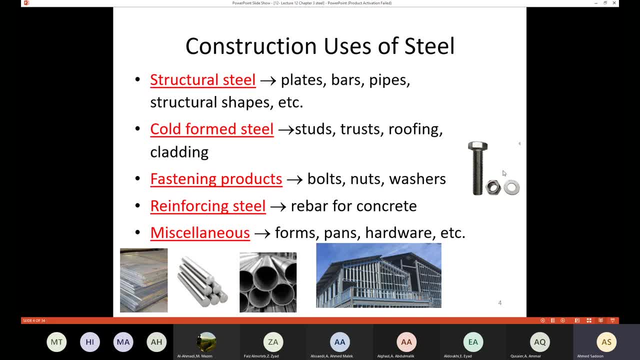 We have the bolt, We have the nut and we have the washer. Also, we have the reinforcing steel, The steel that is going to use for the concrete in order to strengthen the tension capacity. Also, we have miscellaneous like the forms, hands and hardware. 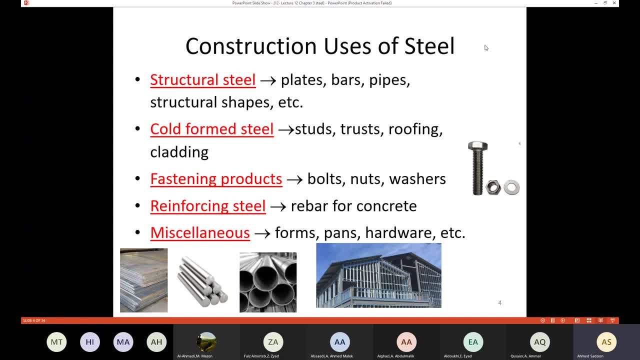 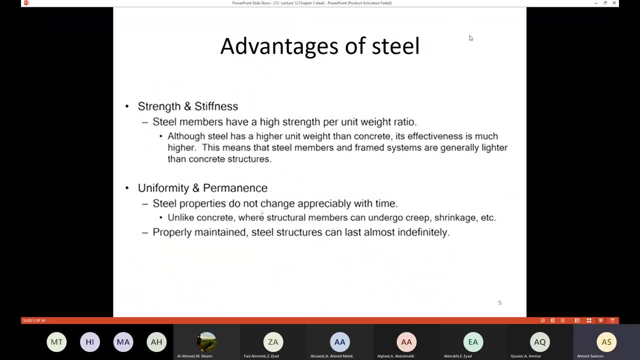 Okay, So we have a different type of steel in construction. Okay, So why we should use the steel? What is the advantages of the steel? First, we have the strength and the stiffness. The steel members have a higher strength per unit weight ratio. 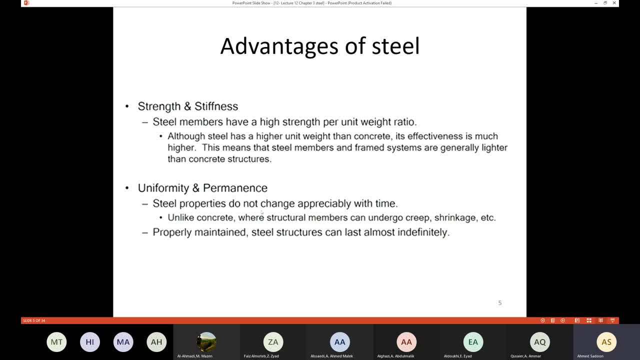 So if you are going to compare the steel with concrete and with asphalt and you are going to determine this ratio, the strength per unit weight, then you are going to have, you are going to get that the steel has a higher strength. 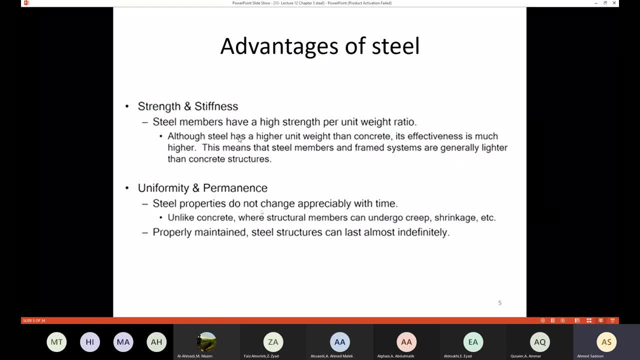 the strength per unit weight ratio. Even though the steel has a higher unit weight than concrete, the unit weight of the steel is lower than the concrete. its effectiveness is much higher. This means that the steel members and the frame system are generally lighter than the concrete structure. 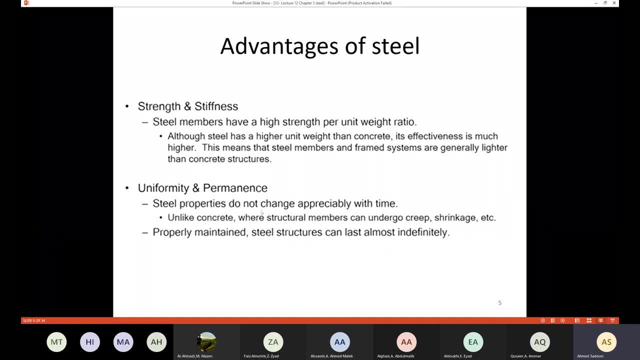 So if you have a frame that made from steel and another frame made from concrete, then the frame that made with the steel is going to be lighter than the concrete, the frame that which made from the concrete. also, we have the uniformity and permanence. 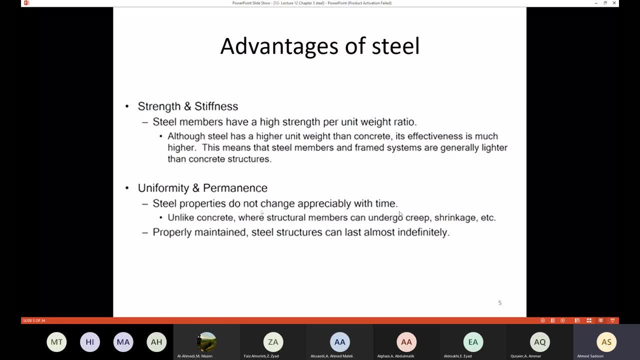 so steel properties do not change appreciably with the time. remember, regarding the concrete, we talk about the creep, about the shrinkage. with the time we are going to have many problems. so all of these problems like the creep and the shrink, does not exist in steel. so the, the, 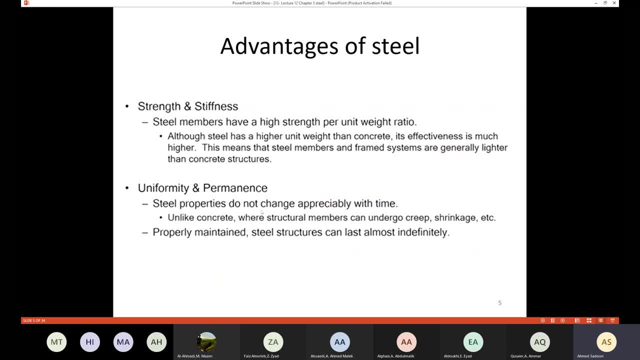 properties of the steel is not going to change with the time, okay. and also, if you are going to maintain the steel in a good condition condition, the steel structure can last almost indefinitely. so for the, the, the steel, it can last forever if you provide good maintenance. okay, if you provide good maintenance, the steel can last for a very long time. 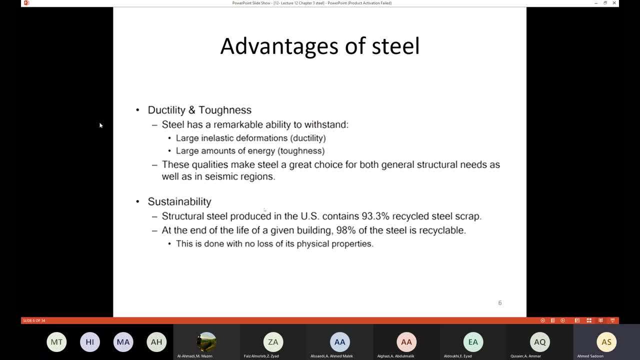 also, we have other proper advantages for the steel, like the ductility and the toughness. the steel has a remarkable ability to to withstand the large inelastic deformation, which means that it has large ductility. we talk about the ductile material and brittle material, and the steel is going to provide. 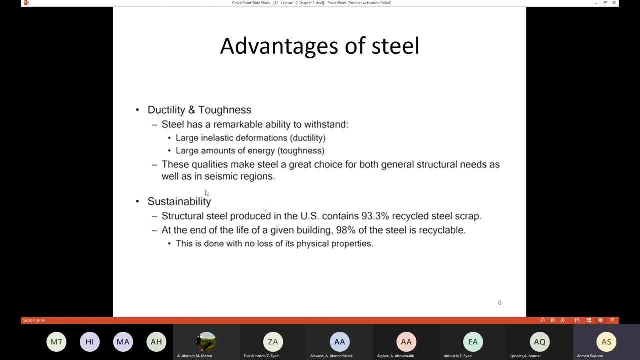 a large capacity of ductility also is going to provide a large amount of energy. the toughness- remember the uh toughness. we managed to determine the toughness. if you have a stress strain diagram, you could be able to determine the stiffness, the toughness. so the toughness of the steel. 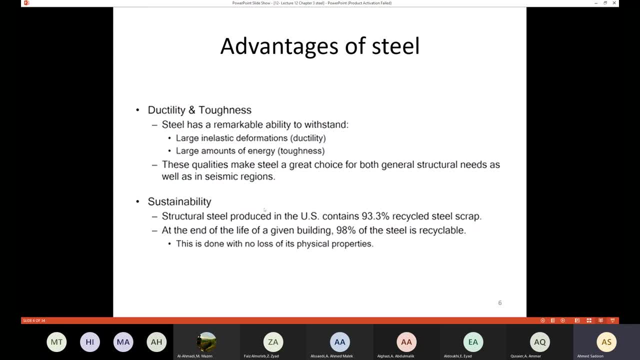 is uh is large. that is going to help us, especially in uh systemic regions. so these qualities- the ductility and the toughness- make a steel a great choice for both general structural needs as well as in seismic regions, when you are going to expect to build a steel structure in seismic regions. 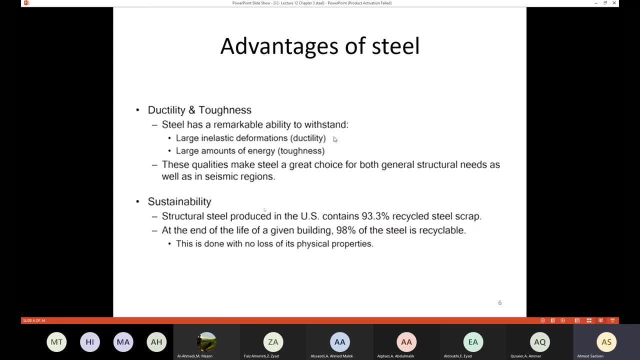 have earthquake. so the the ability and the toughness is a good advantages when you're using steel. finally, we have the sustain: sustainability. structural steel produced in the us contains 93 point three percent recycled steel scrap. so steel it could be recycled on large scale. okay, so at the 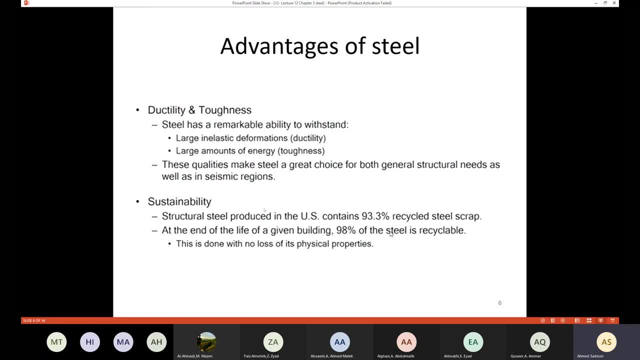 end of the life of a given building, 98 of the steel is recyclable. so if you made a building from the steel, then 98 of all of this steel it could be. uh, you can recycle that amount, okay, and this could be done with no loss of its physical properties. so you can, uh. 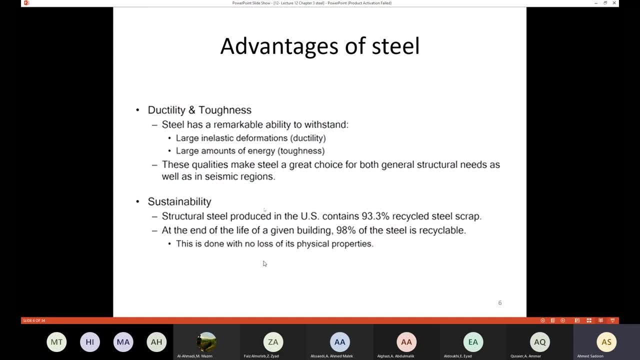 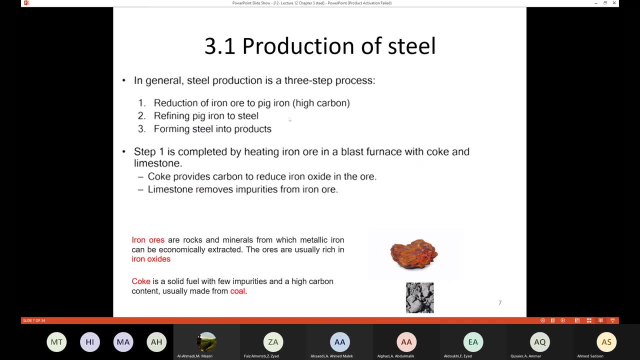 you can recycle the steel without using the physical properties. so in terms of sustainability, using steel is very good. so now we need to talk about how to produce steel. we are going to talk about the production of the steel generally. we have three steps in order to produce steel. we have 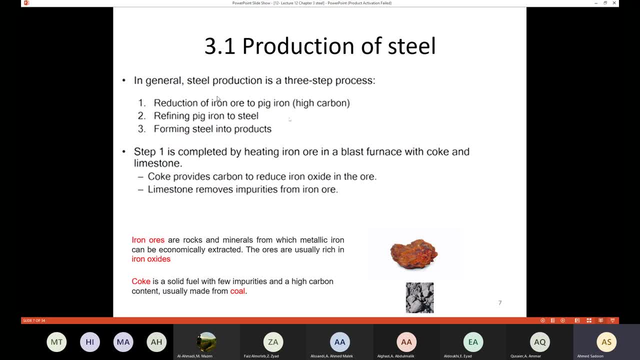 three steps. step number one: the reduction of the iron ore to pick iron, uh the in this one here it's going to be completed by heating the iron ore. here is the iron ore: iron ore in the rocks and minerals from which metallic iron can be economically extracted. the ores are usually. 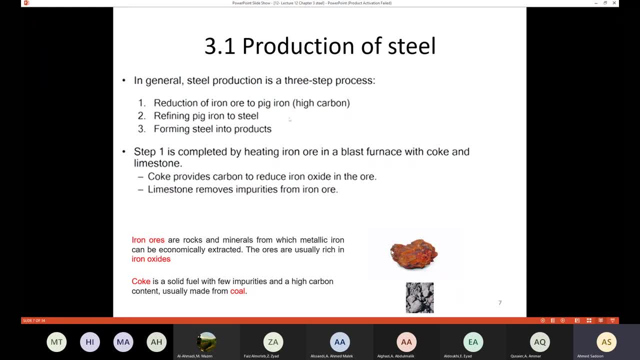 rich in iron oxides. so we are going to first pick up this kind of rocks. we call this iron ores, this kind of rocks rich in iron oxides. so we need to pick up this one here and we need to put this in the uh blast furnace, this one, the blast furnace. i need to put the blast furnace. 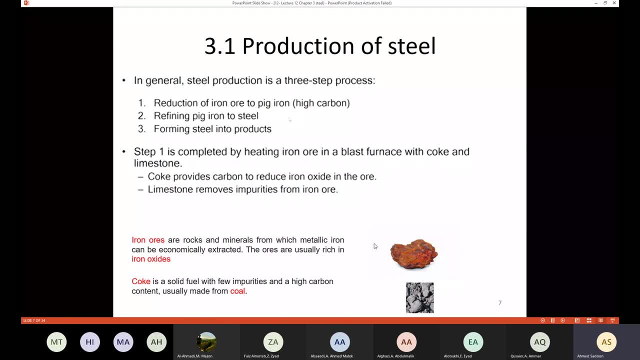 to the uh, the iron ore, and also i need to to use the limestone. i need to use the uh, the uh coke, okay. so i need to have the iron ore, i need to have the coke and i need to have the limestone. so the coke is the solid fuel with a few impurities and high carbon content, usually made from coal. so 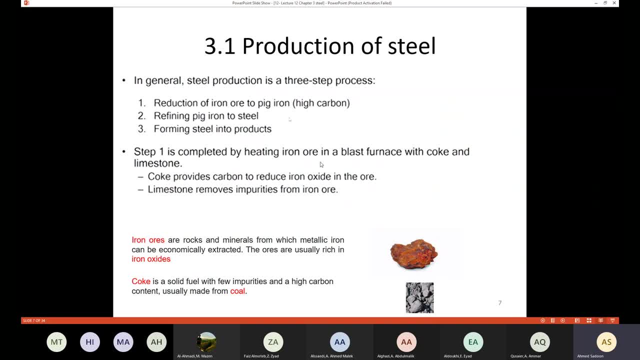 i need to have coke and the limestone, so i will be using the limestone. i need to put the iron ore in the blast furnace and I need to have limestone and I need to have the iron ore. so what is a? what is the purpose of the coke? the coke is going to provide carbon to reduce iron. 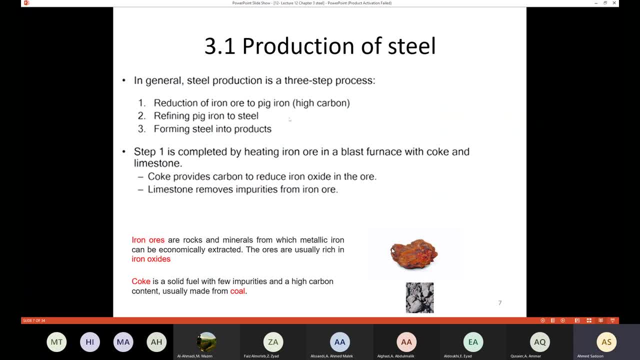 ore in the ore. so here we have the ore. the ore is going to be rich in iron oxide, so the coke is going to provide carbon to reduce the iron ore in the ore. here also we have the limestone. the limestone is going to help us to remove. 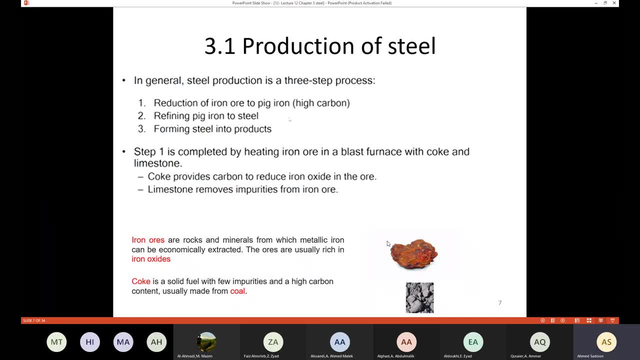 the impurities from the iron ore. so the the basic component is iron ore, but I need to use the coke in order to provide carbon to reduce iron oxide, and also I need to use limestone in order to remove the impurities from the iron ore. so the 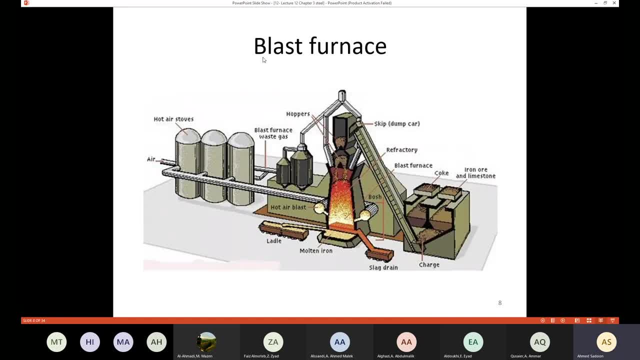 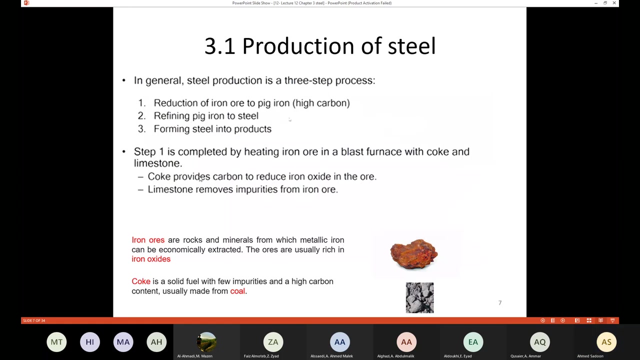 first step here. I'm going to use a blast furnace and I'm going to have iron ore, I'm going to have limestone, I'm going to have coke, okay, so all of this is going to be delivered to the blast furnace with a certain amounts, okay. so we, we've done with the first step. 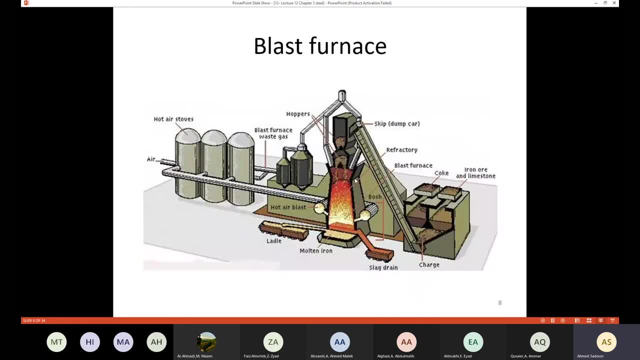 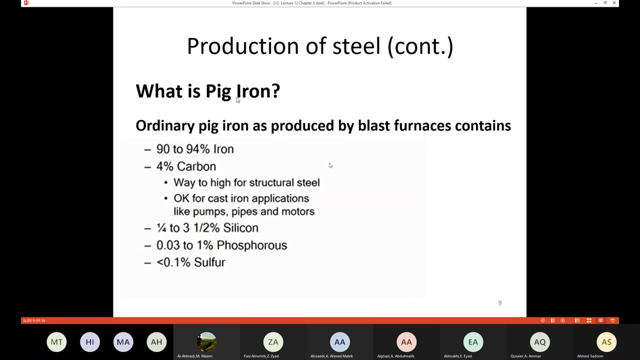 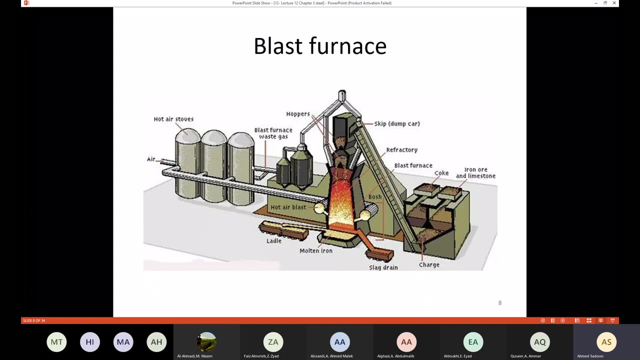 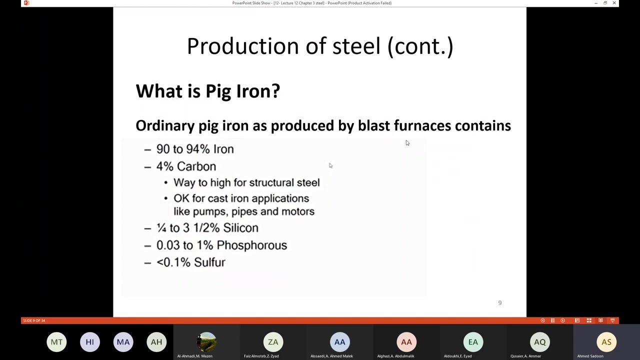 then uh, the, uh, the, the process from step number one we are going to have. we are going to have the pick iron. so the result of mixing the iron ore and the coke and the limestone, we're going to get the pick iron. so the ordinary pick iron are produced by the blast furnace. so from the blast furnace, here the 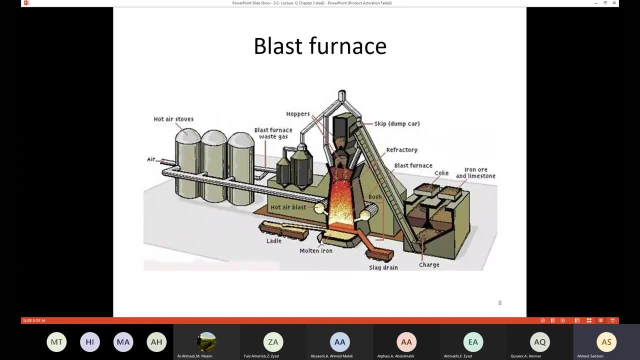 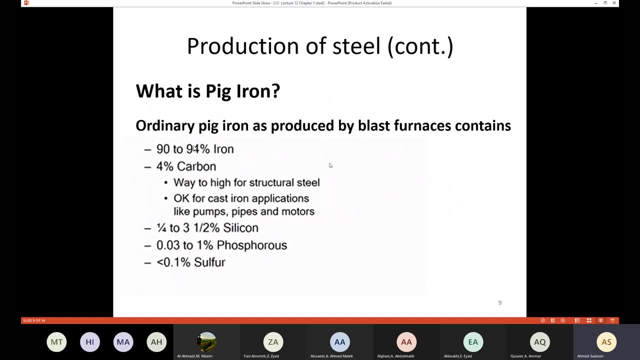 molten iron. here is the, the pick iron. so what is the properties of the pick iron? this one is going to have between 90 to 10 year onions, tong B name is this one- sourced fruits and milk. This one is going to have between 90% to 94% iron. we are going to have 4% carbon, but this percentage here is way too high for structural steel. 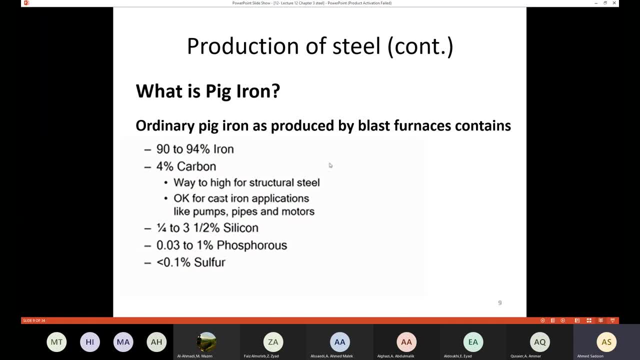 It could be used for cast iron. Usually the cast iron. we made the machines and so on from the cast iron, while the structural steel is the steel that should be used in the structural purposes, The cast iron, like the bumps, like the pipes and like motors, in those we are going to use cast iron and the percentage of the silicon between 1 over 4 to 3.5% and the phosphorus between 0.03 to 1% and the silver is less than 0.1%. 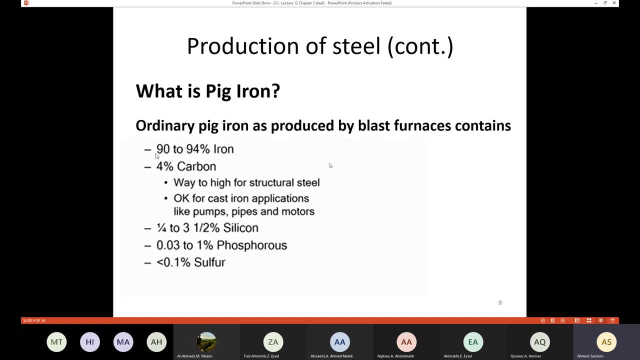 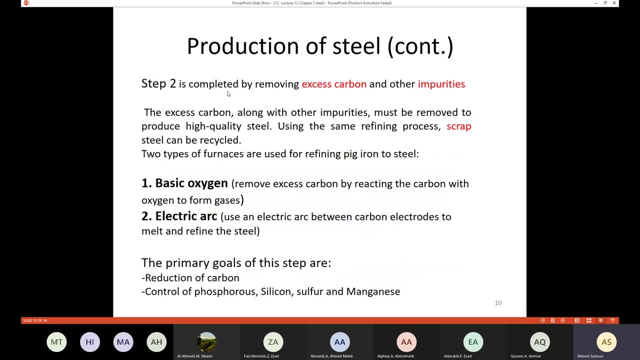 So here is the properties of the pick iron. The problem with the carbon. we need to reduce The percentage of the carbon if we are going to produce structural steel. So in this step, this step should be completed by removing excess carbon and other impurities. 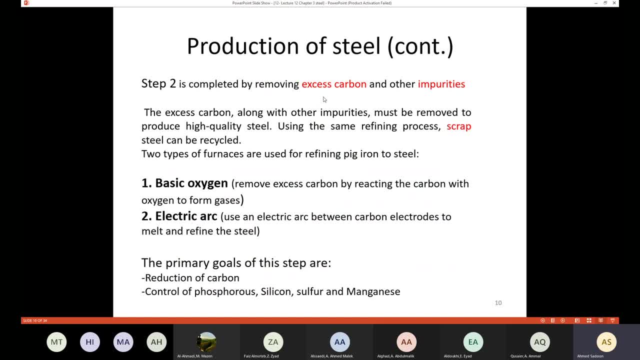 So in this step, I'm going to remove the excess amount of carbon and also I'm going to remove any impurities. So the excess carbon, along with the other impurities, must be removed to produce high quality steel. So, in order to produce high quality steel, you need to remove the excess carbon and also you need to remove the impurities. 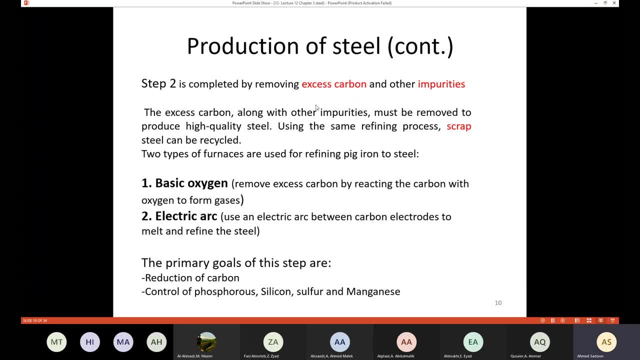 And the same process. it could be used for scrap in order for the steel to be recycled. Scrap is the remaining of the steel, So the same process. it could be used for scrap for recycling processes. So we have two types of furnaces. 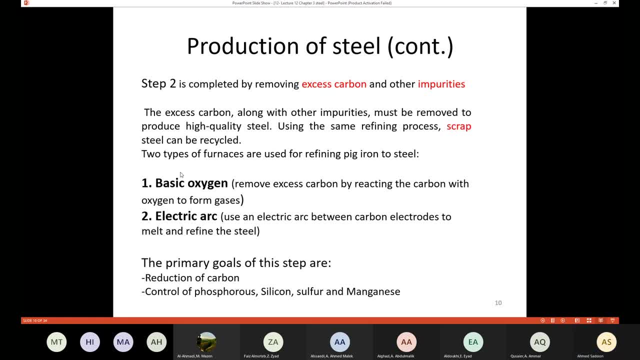 They are used for refining pick iron to steel, Either to use the basic oxygen or to use the electric arch. In both methods we are going to remove the excess carbon In the basic oxygen. we are going to remove excess carbon by reacting the carbon with the oxygen to form gases. 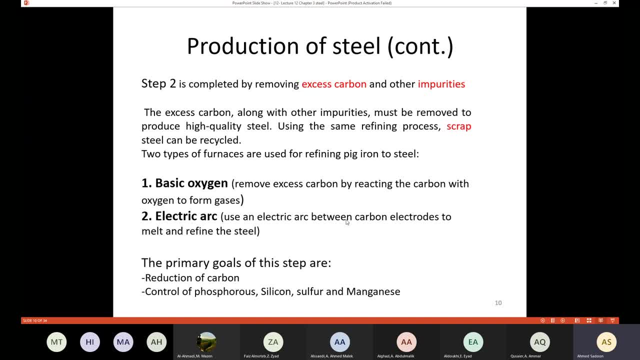 While in electric arch, we are going to use an electric arch between the carbon electrodes to melt, And then we are going to use an electric arch between the carbon electrodes to melt, And then we are going to use an electric arch between the carbon electrodes to melt. 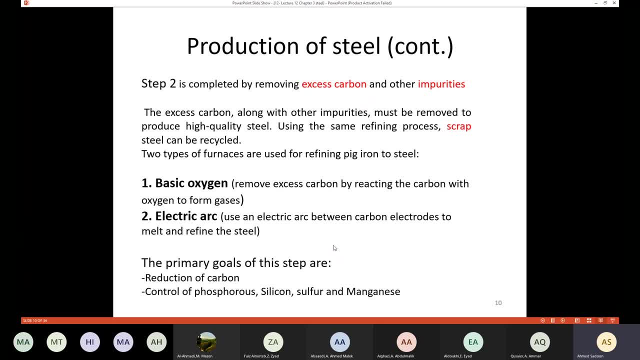 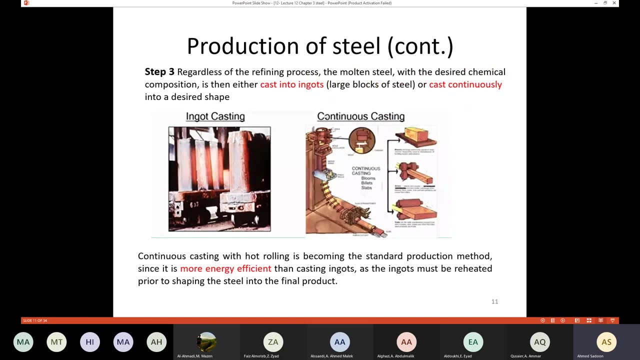 We multimodally refining the steel. You can use this one and that one, But the primary goal for this step is reduction of the carbon and the control of the physics: silicon, silver and magnesium. So the last step instead number three: ah, regardless of the refining process. 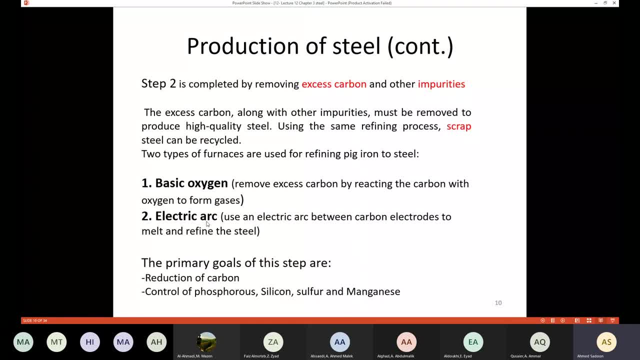 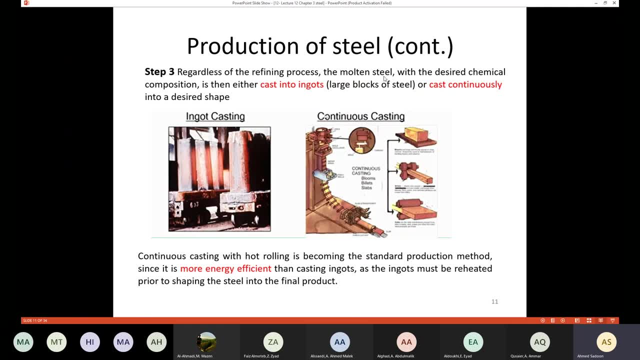 whether you are going to use the basic oxygen or electric arch in order to remove the access carbon and the impurities. uh, the molten IVF, the molten steel with the desired chemical composition, is then either cast into ingots, which is a large block of steel- then we are going to put the steel like that in a large blocks, or 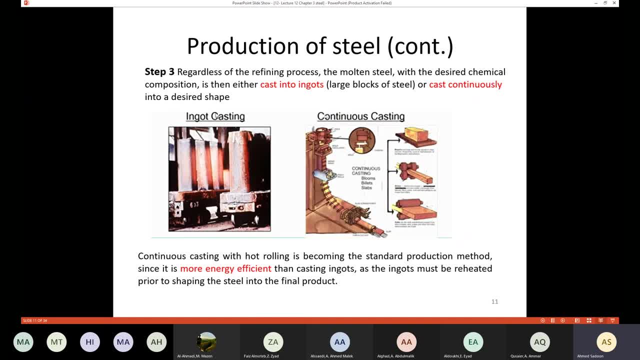 it can continuously. it can cast continuously into desired shape. so once i got the steel, once i got the molten steel, i have two options: either to put them as ingots in a large block, or i'm going to directly cast the steel in desired shape using the continuous casting. so i'm going to place the 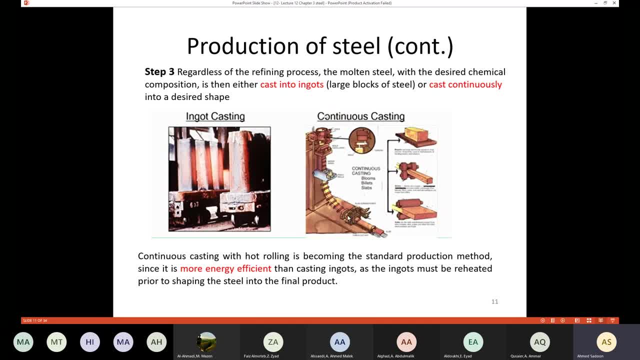 concrete to go through this process of rolling so that we can shape the concrete into the desired shape. so now, continuous casting. this one is a continuous casting. i'm going to produce directly, i'm going to produce steel in desired shape using the continuous casting. with hot rolling is becoming the standard production method. so nowadays no one is going to 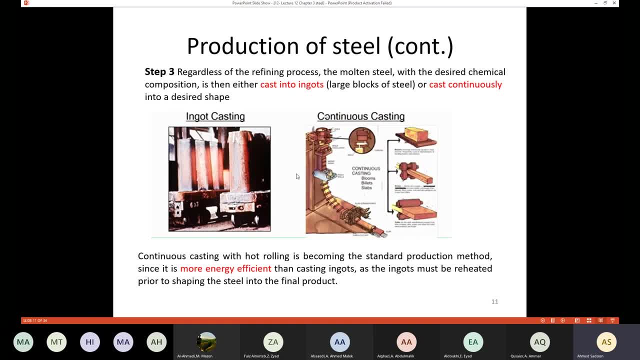 put the steel in ingots. okay, the standard. now we are going to directly produce the steel in desired shape using the continuous casting and the hot rolling. why we do that? because it's more energy efficient than cast ingots. because, like you can see here in the ingots i need in order 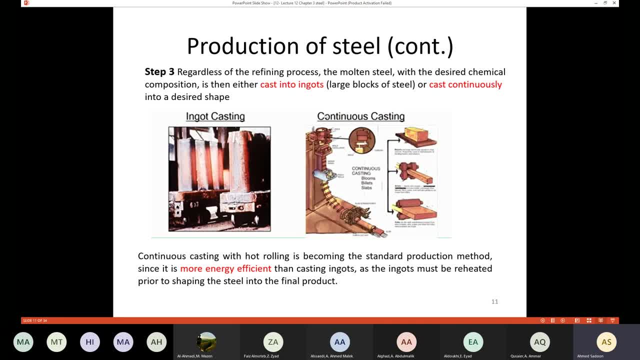 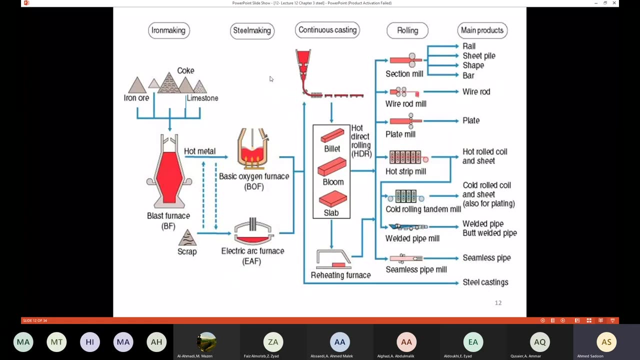 to to get my desired shape. i'm going to reheat the- uh, the ingots again so that i can get my desired shape. so this one is going to consume more energy than the continuous casting. here we have a graph that can summarize the process. uh, first i need to have iron ore, and also i need to have a coke and i need to have 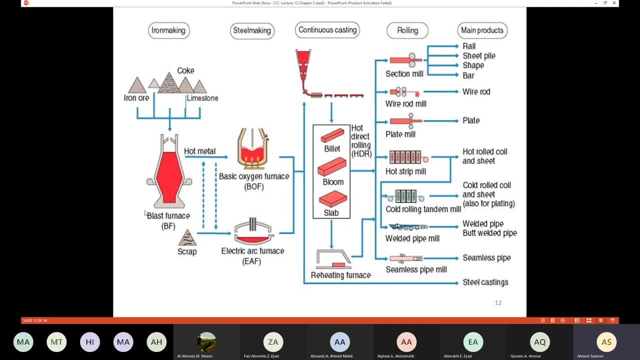 limestone, so i'm going to put them in the blast furnace. okay, then i'm going to have the molten steel, the hot metal, okay, so, uh, now i'm i'm done with the step number one. i'm going to have the pick iron, which is rich in carbon, and also you have, uh, some impurities. 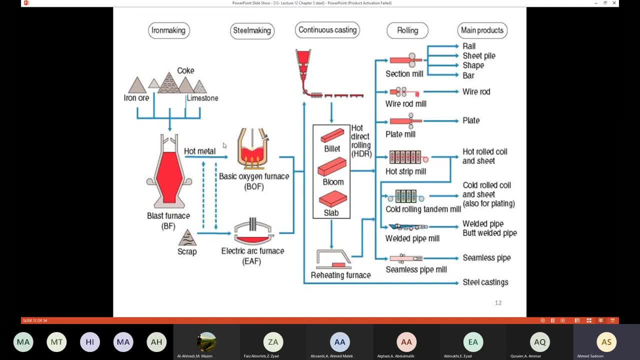 impurities. in order to get rid of the excess carbon and the impurities, either to use the basic oxygen furnace or the electric arch furnace. The same step here: if you have scrap, if you have remaining of steel, you are going to use the basic oxygen furnace or the electric arch. 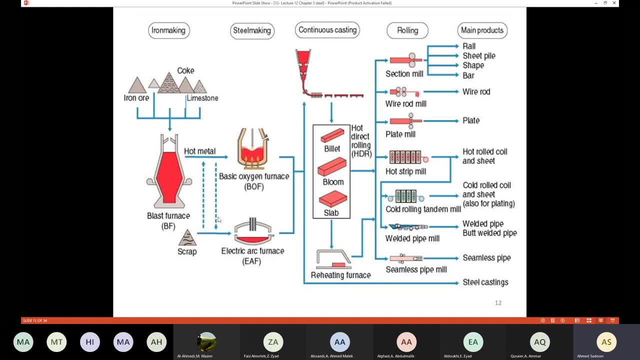 furnace, Like we just mentioned. regarding the scrap, we are going to use the same method. We are going to start from step number two. After that we are going to put the steel in the desired composition. Then I have two options: either to use the continuous casting- this one- or I can. 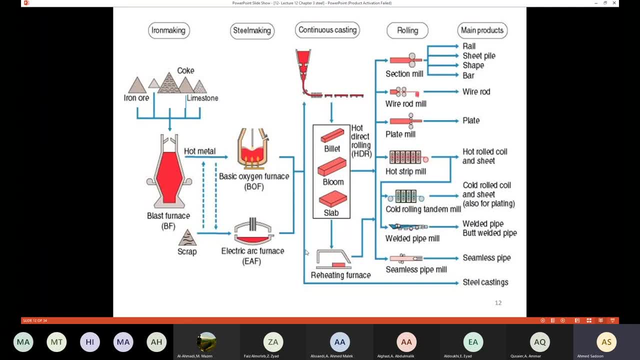 put the steel in the ingots. If I'm going to put the steel in ingots, then later on I need to reheat the steel again so that I'm going to continue the rolling process. So here I'm going to use the continuous casting, I'm going to put the steel 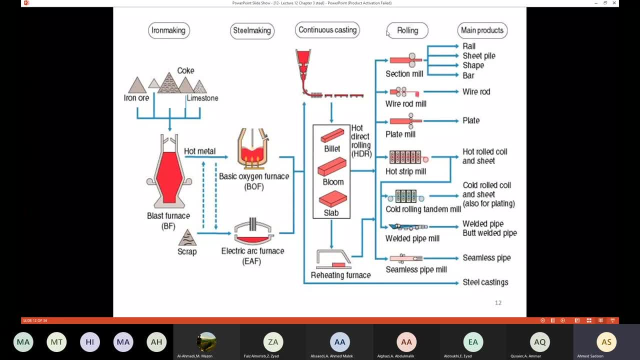 in shape like this one or this one, or like that one, and then it's going to go through the rolling. This one rolling is going to control the shape of the steel and then I'm going to have the products, whether you are going to have rail, sheet, tile shape, bar, wire, rod blades. 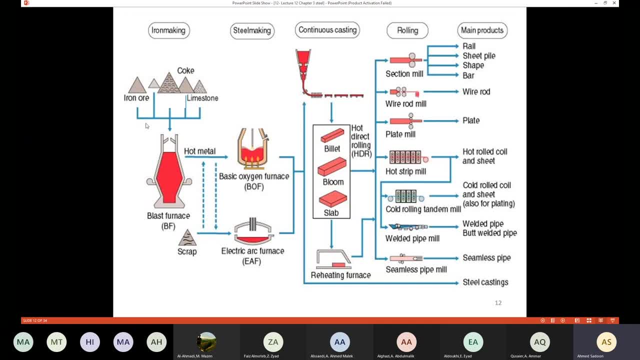 all of this is the final products. Okay, so here I have the blast furnace, the first step. Then I'm going to have the second step, the basic oxygen furnace, an electric arch furnace, Then I'm going to have the continuous casting. 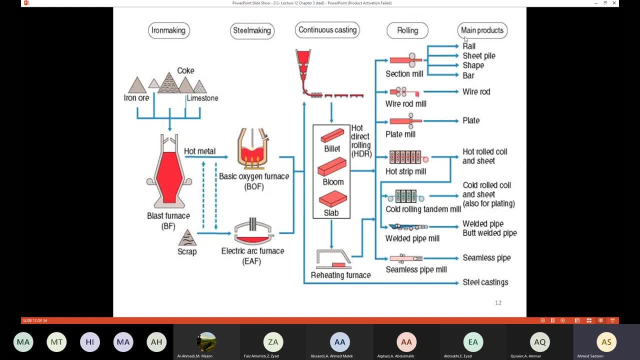 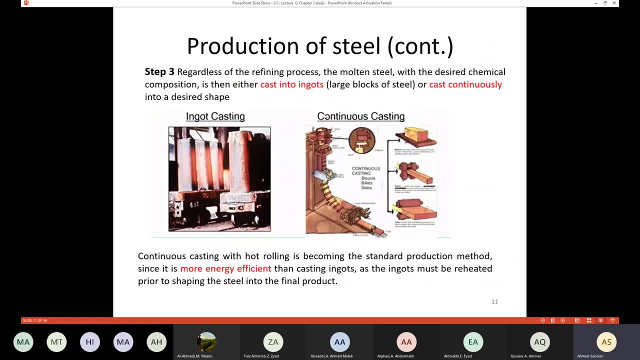 Then I'm going to have rolling process and finally I'm going to have the main products. So now we have a good idea about how to produce the steel. We say that as civil engineers we do not specialize in steel production. We say that we are going to use the steel in the 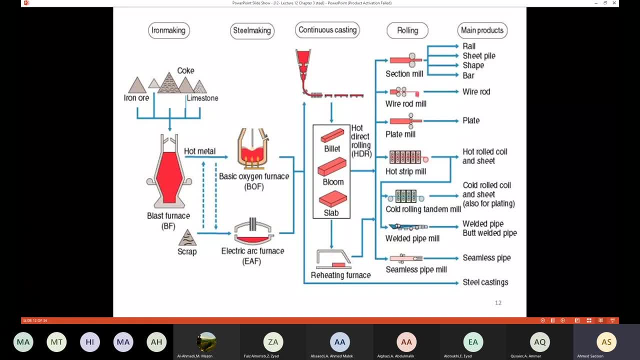 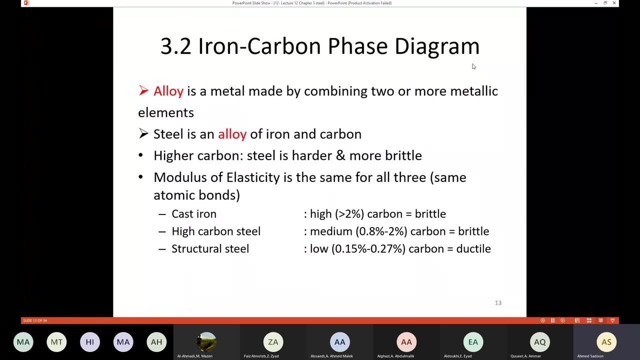 process. We do not specify the properties of the steel, We do not specify the strength or the durability, but we need to understand the process. That is going to help us a lot. So now we need to talk about the iron carbon phase diagram. 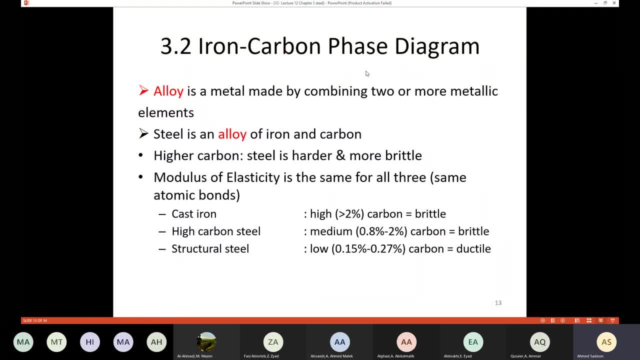 Okay, The percentage of the carbon is going to control the behavior of the steel. Okay, So if the percentage of the steel it more than two percent percent, the steel is going to be brittle. we are not going to have ductility and also in the 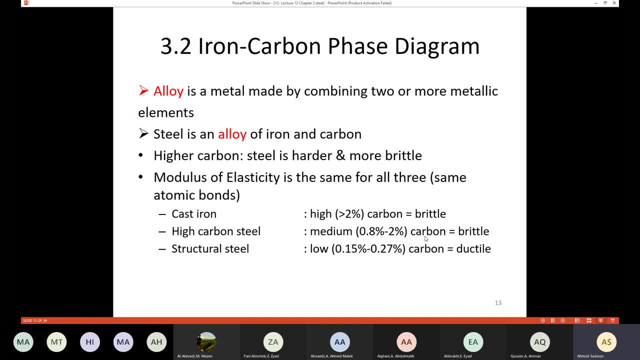 percentage of the carbon between 0.8 and 2 percent. again the carbon, the steel, is going to be brittle. if the percentage is more than two, we are going to call the steel cast iron. if it's between 0.8 percent and two percent, we are going to call this high carbon steel. and also the behavior is brittle. 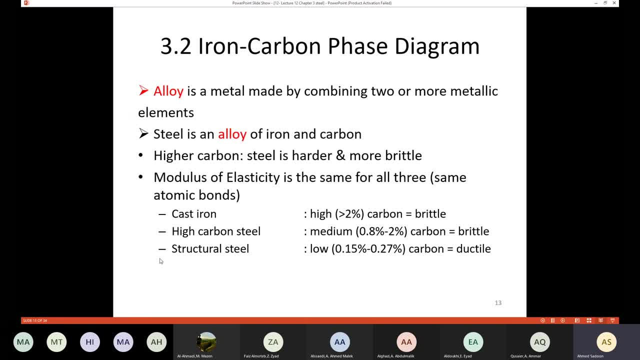 and finally we have the structural steel, which is we really want to use, uh, the. the percentage of the carbon is going to be low, between 0.15 percent to 0.27 percent, and this one is the ductile. this one, it have a better ductility than the cast iron and high carbon steel. we call this iron carbon. 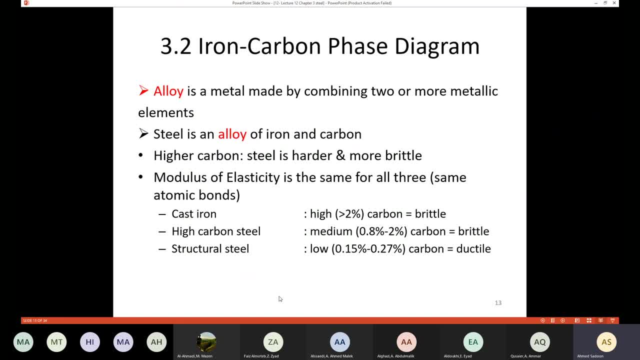 phase diagram. so the, the percentage of the carbon, is going to control the behavior of the steel. you also we have the alloy. we say the, the term alloy for a metal made by combining two or more metallic elements. so if you have a metal that it has been produced by combining two or more elements, we call 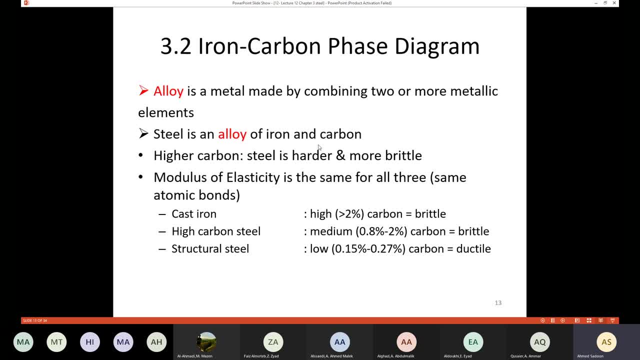 steel is iron, have carbon. the carbon is going to show me the behavior, or it's going to control the behavior of the steel, and the carbon is going to control the behavior of the steel and the carbon of the steel, whether you have cast iron or high carbon steel or structural steel, the behavior here. 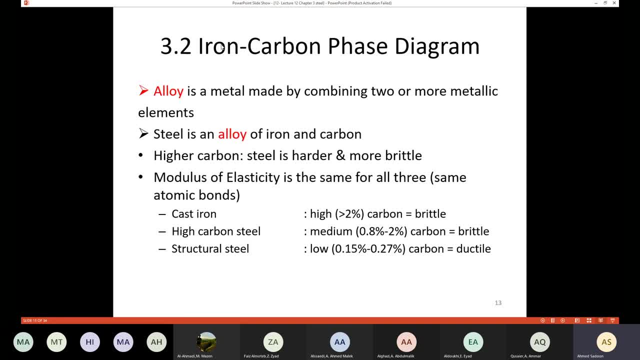 is going to be different, but you need to remember that, whatever the percentage of the carbon, the modulus of elasticity is the same for the all three because they have the same atomic bonds. so i'm always asked about this. so please remember that, whatever the percentage of the carbon, the 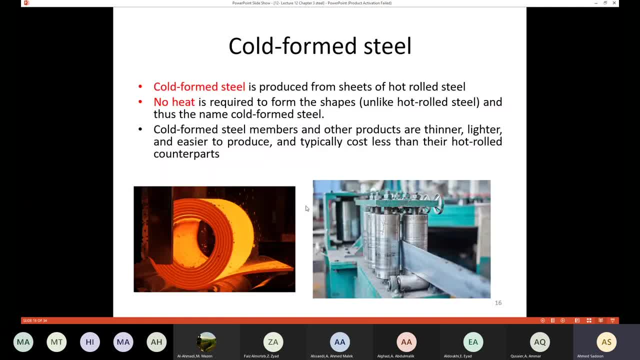 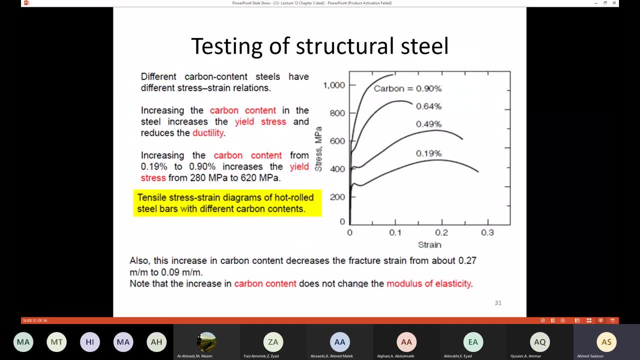 modulus of elasticity is going to be the same, for example. here i'm going to jump to this diagram so that you can understand this. so here we have steel. we have uh stress strain relationship for steel with a different percentage of the carbon. so here we have this percentage i have 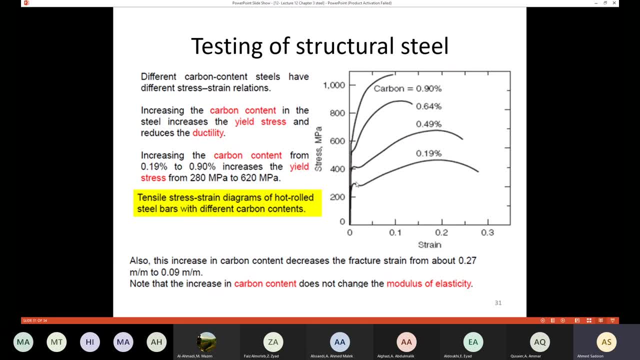 this percentage and have this presenting and that percentage so you can see here when i'm going to use the percentage of the carbon, because as you can see in the figure to our second picture of the carbon, the behavior is going to be more dictile If I'm going to increase. 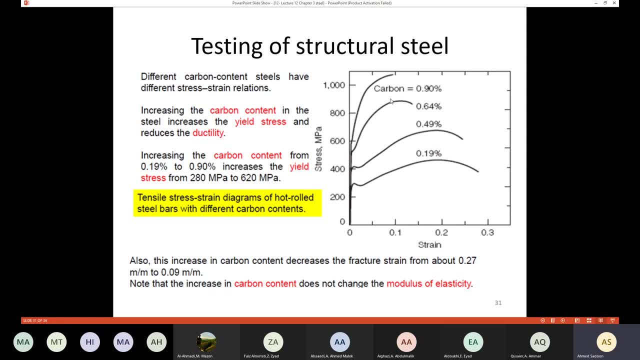 the percentage of the carbon. the behavior is going to be more brittle, even though the strength is going to be better, but the volatility is going to be less. But here, if I'm going to measure the slope, here, the modulus of elasticity. 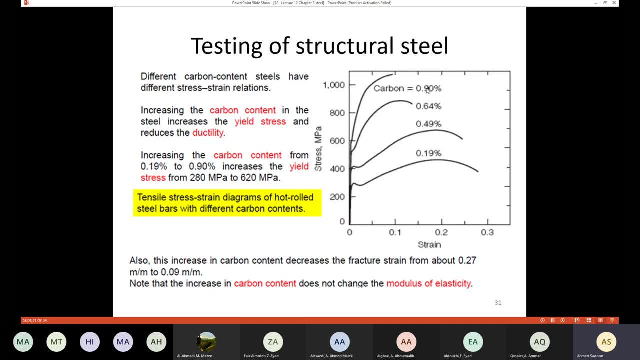 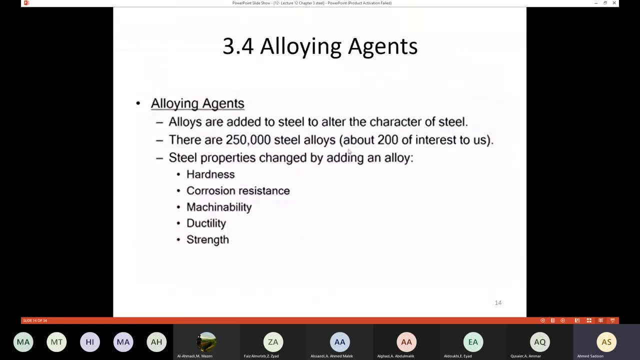 the modulus of elasticity is going to be the same for all steel, whatever the percentage of the carbon. So you need to understand this point. So we have allowing agents- So we said that all of these are added to steel- to alter the character of. 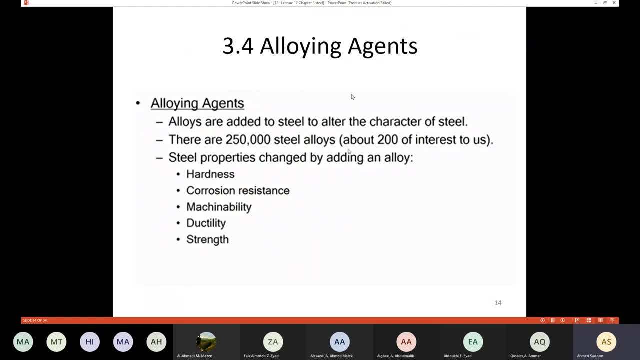 the steel. So here we have something similar to the admixtures in concrete. Here we have allowing agents. This is going to be added to steel so that we can change the character of the steel. They are 200 and 50,000 steel alloys. 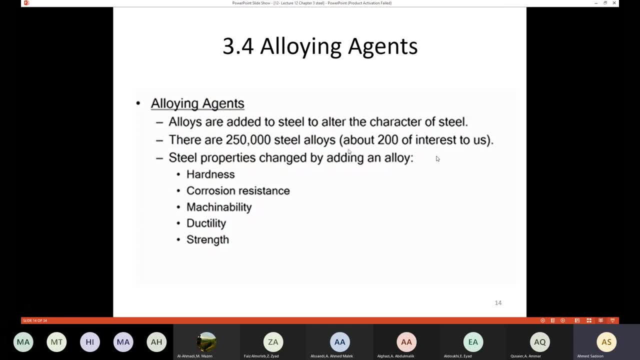 Only 200 is of interest to us. So by adding steel alloys, the steel properties could be changed. You could change the hardness, You could change the corrosion resistance, You could change the mechanability, You could change the ductility and you can change the strength. So by 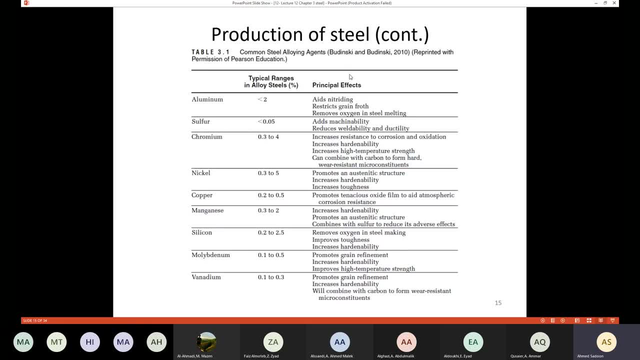 adding the allowing agents. Here we have example for that. If the percentage of the aluminum is less than two, then you are going to, for example, remove oxygen in the steel melting. You could have eights in the trading. You can restrict grain. 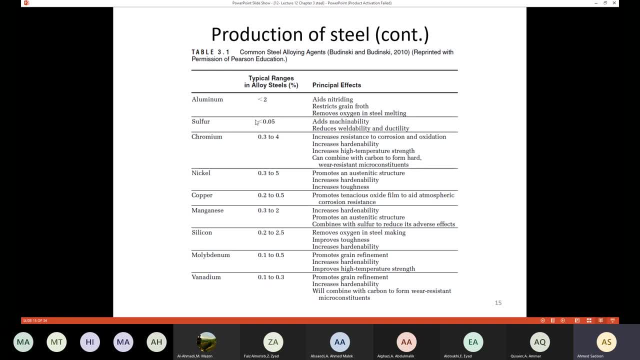 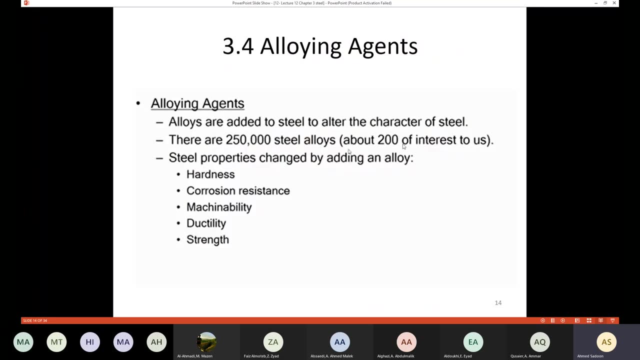 forth. For example, if you have a silver, if it's less than 0.05, then you can add mechanability, You can reduce the ductility, and so on. If I nickel copper, all of this is going to influence the behavior of the steel. This table is. 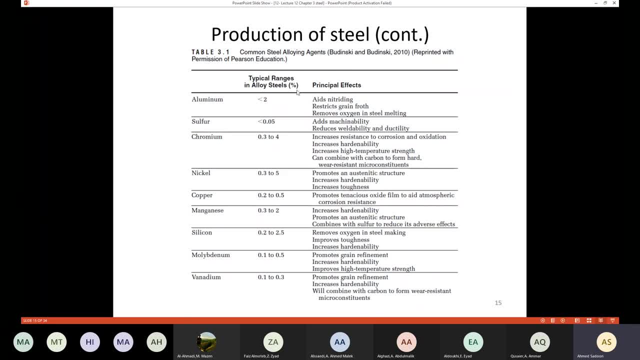 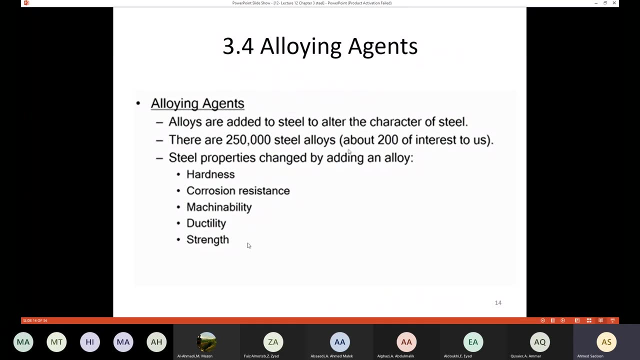 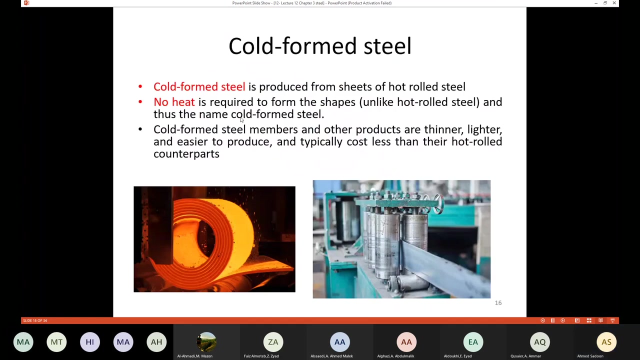 not for for you to memorize, Just to understand that you have allowing agents that can alter the behavior of the steel. Okay, so you can alter many properties like the hardness, corrosion resistance, mechanical ability, ductility and the strings. Also, we have the cold form steel. Okay, the 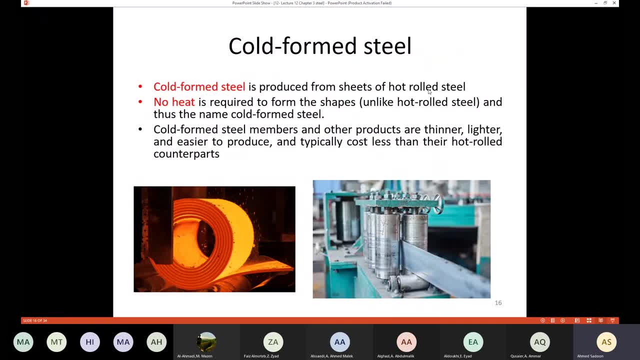 cold form steel is produced from sheets of hot rolled steel. so when we say that cold form steel, this one is going is produced from a hot rolling steel, so everything, everything is going to be produced from, from hot rolling steel. so here we have the hot rolling steel. we could produce the 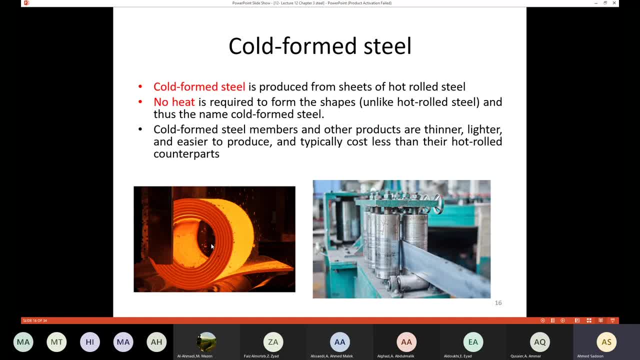 cold form steel, then we are going to store the cold form steel later on. we are not going to use heat, but we are going to use only these machines like this one in order to change the shape of the of these sheets. so no heat is required to form the shapes, unlike hot roll steel and thus name. 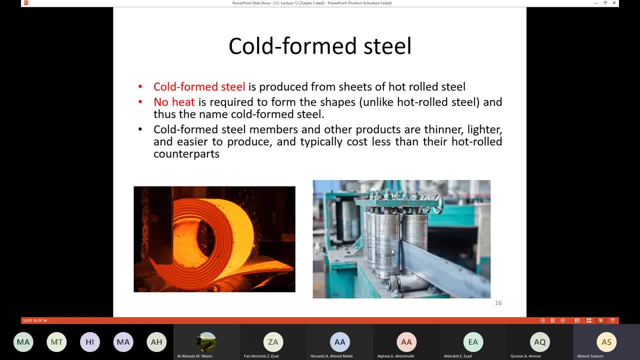 cold form steel. so in order to get the final product for the cold product, we are going to use these machines like this one in order to change the shape of the steel sheets so the cold form steel members and other products are thinner. these products thinner and lighter and easier to produce and typically cost less than. 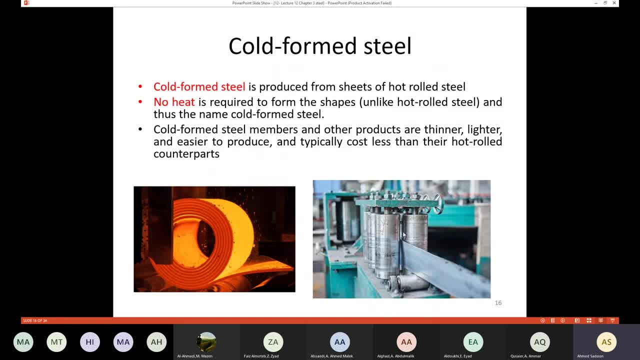 their hot roll counterparts. so this one is going to be shaped using no heat, using only this machine. they can produce honestly liquid metal. own looks like you and when you store Muslim to use these both. probably its cheap, but be apart and does not mean used for theIRE incident. 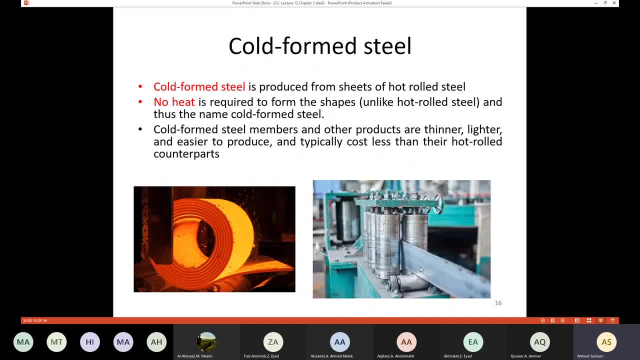 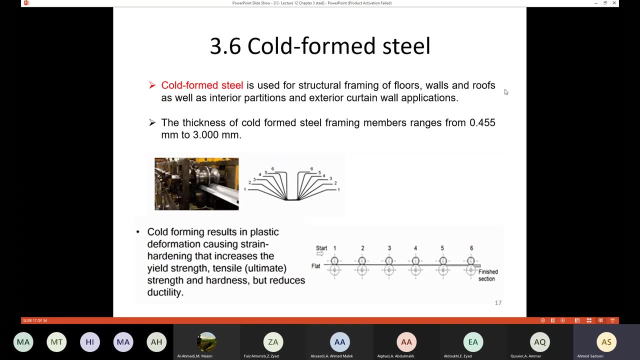 probably theIRE incident or the digital one, because the tip for the human being is to avoid this. machines here and the weight is lighter and the thickness is thinner and they are easy to produce. So the coal-formed steel is used for structural framing on the floor and on walls and on roof. 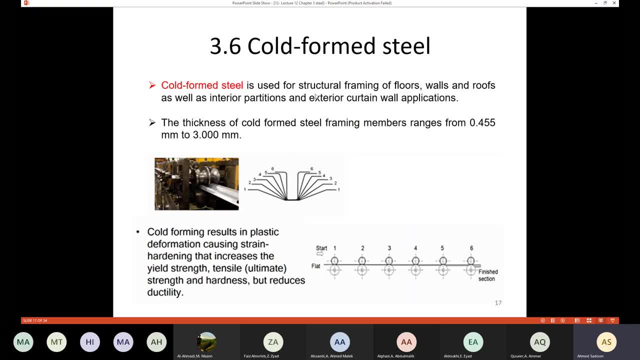 as well as interior partitions and exterior curtains, wall applications. The thickness of the coal-formed steel framing members range from 0.455 millimeter to 3 millimeter. So here we have the machines. help us in order to produce the coal-formed steel And this process. here the 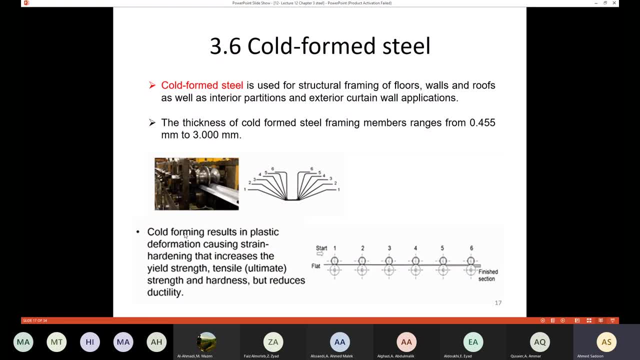 process of forming the steel using these machines result in plastic deformation. We are going to have plastic deformation and that is going to cause strain hardening, That is going to cause stress and that is going to increase the yield strength, the tensile and the strength of the 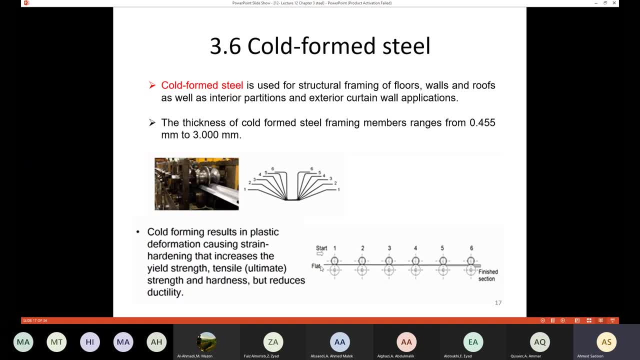 harness, But this one is going to reduce the ductility. So the steel is going to. the steel is first going to be flat, Then it's going to go through those rolling here and then this one is going to be made to produce a desired shape. So the steel is going flat in the beginning, then it's. 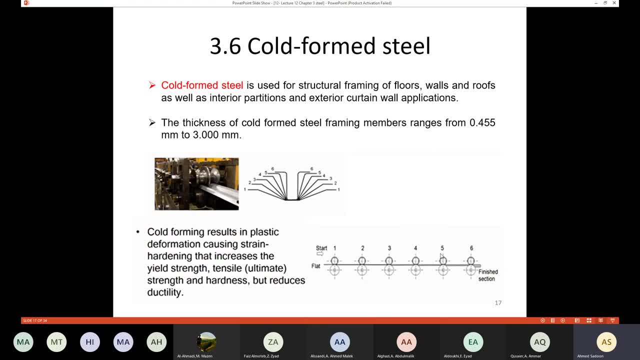 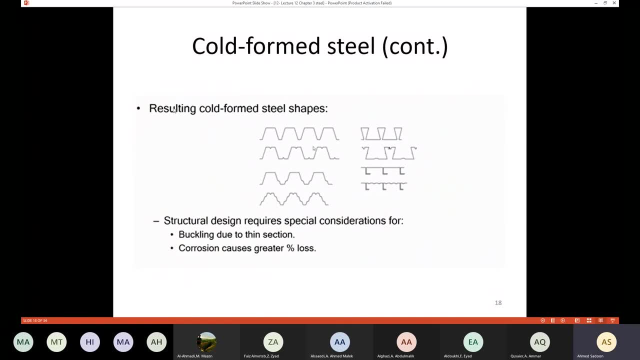 going to go through those rolls rollers and then the finish section is going to be like one of these. so here we have a resulting core form steel shape. the shape could be like that or like that, or like that, or like that. so we have a special consideration for the cold form steel. you need to take care of the buckling. 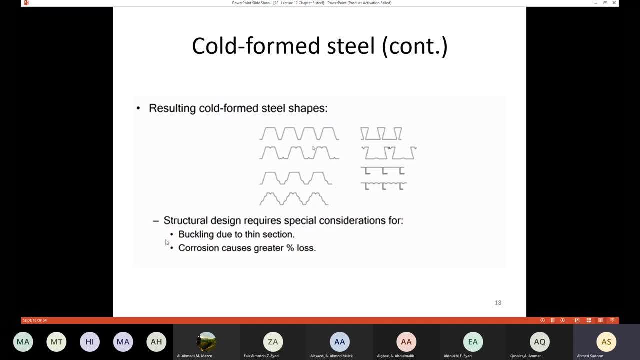 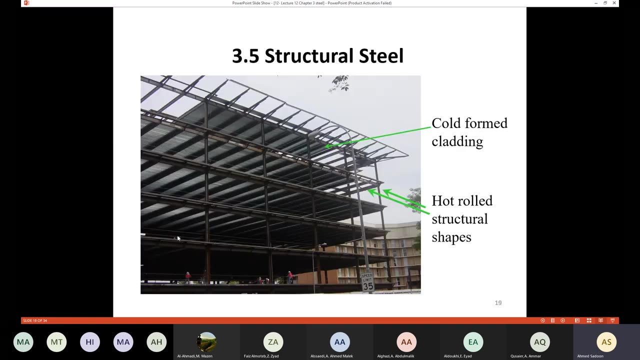 because you have thin section and also you need to. you need to take care of the corrosion, because this one, since the thickness is thin, is going to be susceptible to corrosion. so we need to take care of the buckling and the the corrosion itself. so i'm going to stop here. finally, we have a structural 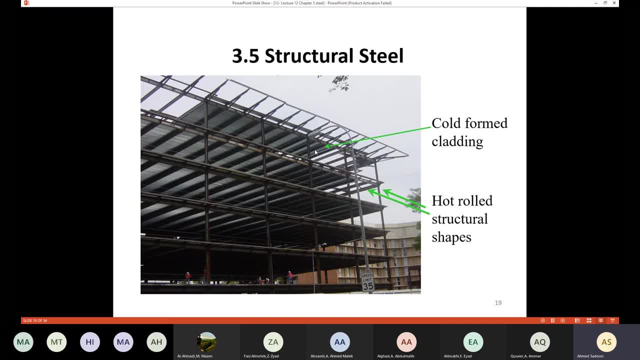 frame. so the cold form, like the cladding and the floor is going to be, is going to place here, like this one for flooring or cladding, while the hot rolled structural shape, like the beam and the column, is going to place here. so in order to come up with or in order to construct a framing steel frame. 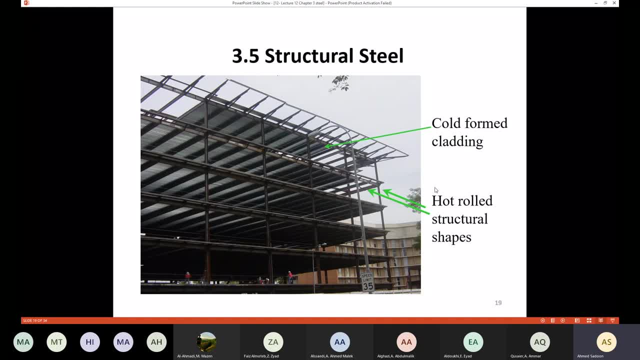 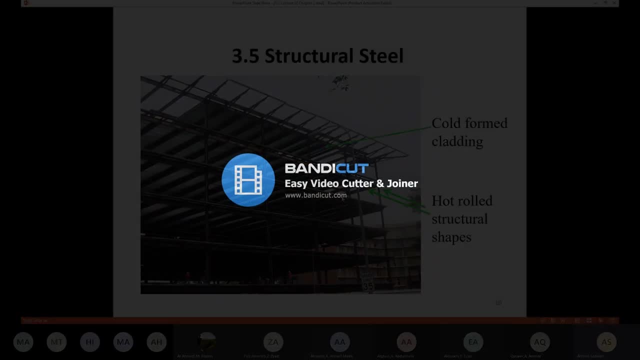 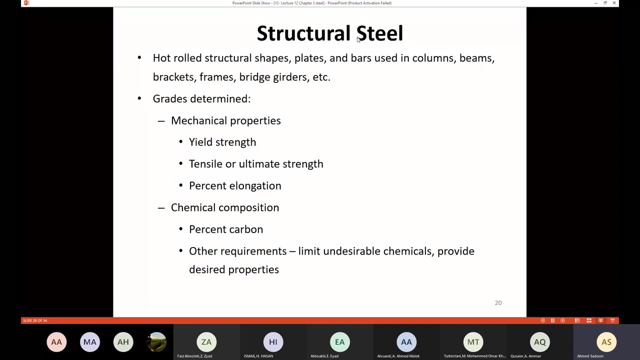 you are going to have cold form steel and you are going to have hot rolled steel, okay, so it's very important to understand where to place the different type of structural frames. so we are going to talk about the mechanical properties and the chemical composition of the structural steel when the structural steel is hot rolled, which means that we are going to 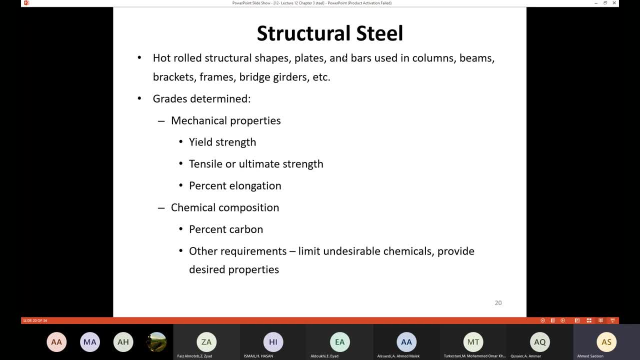 produce shapes, plates and bars and all of this. you are going to use them in columns and beams and brackets, frames and bridge girders. okay, so the hot rolled structural shapes, plates and bars, we are going to use them in columns and beams, for example. but we the the, the, the columns and the beams and all of this. they are graded. 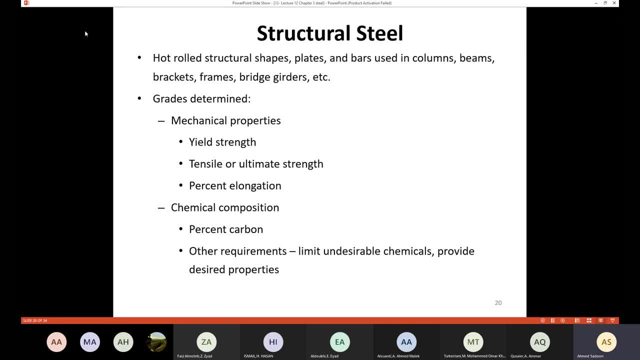 we have grids for them and through the, the grading, we are going to know the mechanical properties and the chemical composition. so what do we expect in the mechanical properties? in the mechanical properties, we are going to know the yield strength. remember the value of the yield strength is the value in the material that differentiate between the elastic and the plastic. 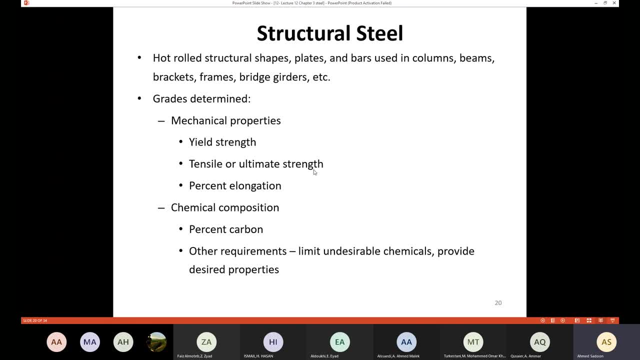 behavior, and we have the tensile, or the ultimate strength, the maximum strength on the curve, and we have the percentage elongation, how much the steel has been elongated after the failure, and also we'll learn how to get all of this through the laser of the machining process. 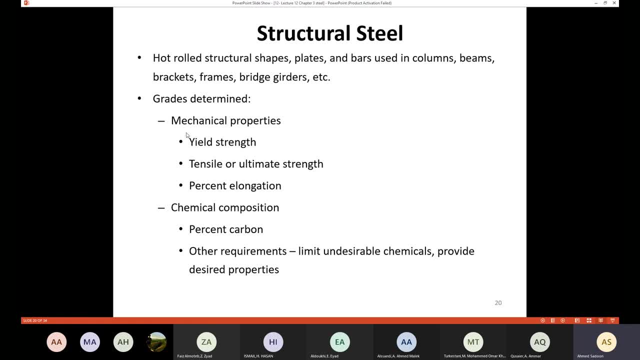 the flaviation process. In lab number eight, when we had the tensile test, we learned how to determine the yield strength, the tensile or the ultimate strength or the percentage elongation. Also, we have the chemical composition. In the chemical composition we'll be able to know the percentage of the carbon. 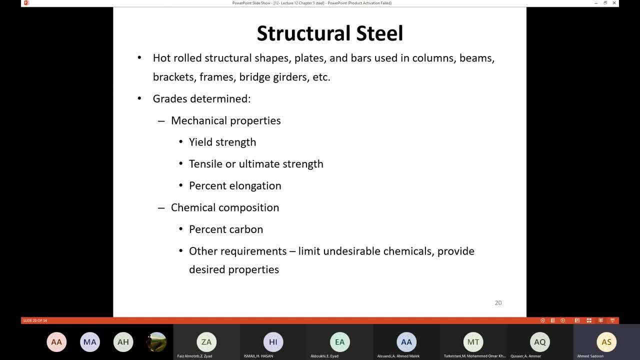 Now we know the role of the carbon in the behavior of the steel. And also we have other requirements, because in the other requirement- limiting undesirable chemicals- we're going to provide desirable properties. So if you are going to limit some chemical, then you are going to improve the desired properties. 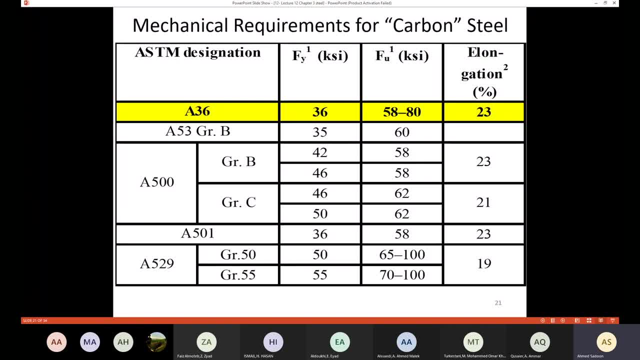 So let's see an example on the grading of the structural steel. So, according to ASTEM, we have many grades here. the most used one is A36, but also we have A53, Grade B and we have 8500, we have Grade B and Grade C. 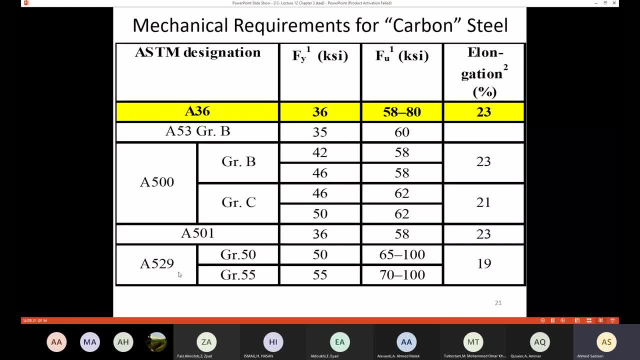 We have A501, we have A529, we have Grade 50 and Grade 55. So here, first we are going to look at the mechanical properties. We are going to know the value of fy, The yield strength of the material. 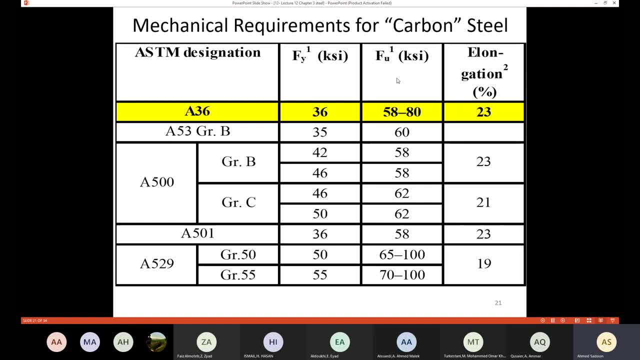 strength, the value of fu, the ultimate strength, and the elongation: how much the element has been elongated after the. so, for example, look at a 36. the value of fy came out to be 36 ksi. so this one is the, the value of the yield strength, the point at which the, the behavior of the material, is going. 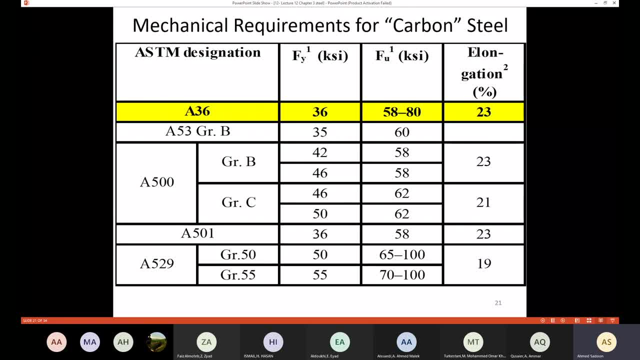 to be plastic behavior, which means that after that value we are going to have permanent deformation. here we have the value of fu, the ultimate strength. it has a range between 58 to 80. so this one is the maximum strength the material can withstand. and here we have the elongation. 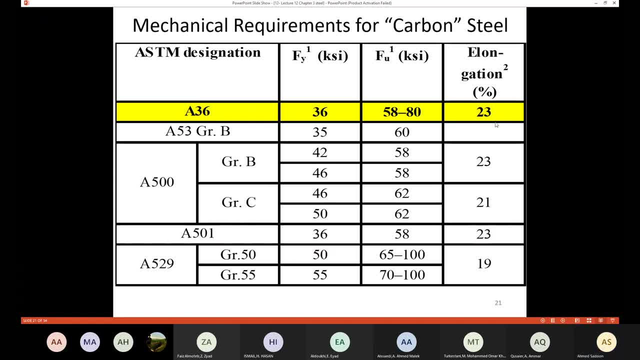 the elongation here is 23 percent, which means that the final length minus the initial links over the initial links is going to give me as a percentage is going to be 23 percent. similarly, here we are gonna know: if you know the, the grade of the steel, then you will be able to know the value of fy. 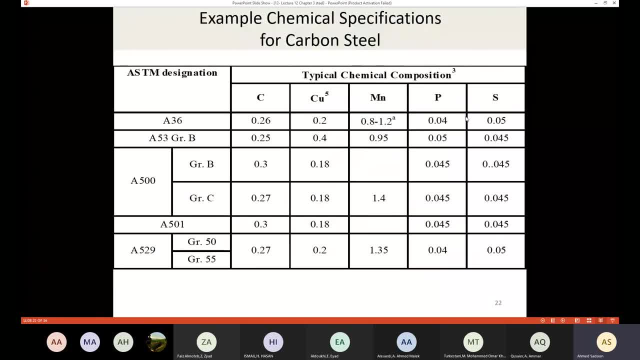 fu and the elongation. similarly, we are going to do the same thing regarding the chemical composition of the material. we are going to do the same thing regarding the chemical composition again, if we are going to have a36 here, the percentage of the carbon, the percentage of. 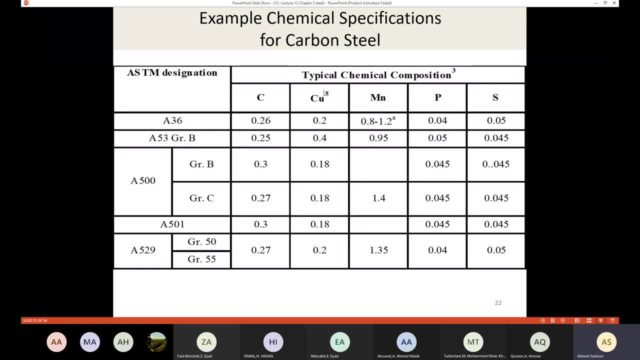 the carbon is 0.26. here we have the percentage of the copper, here we have the percentage of the magnesium, phosphorus and silicon. so here also we are going to know the value of the chemical composition, the value we talked about the importance of the percentage of the carbon. 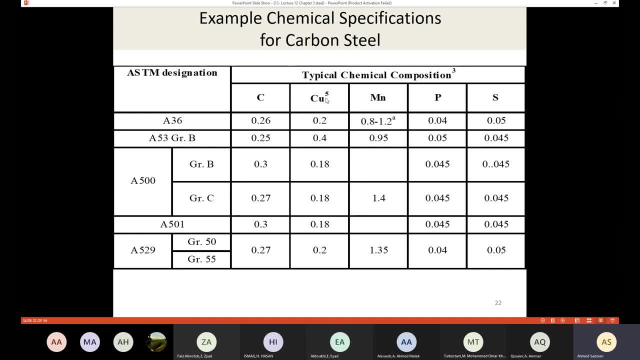 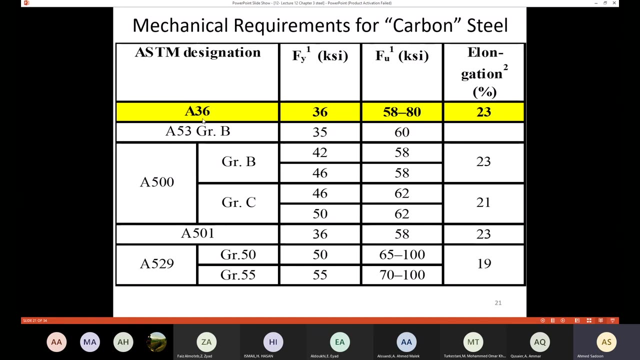 and those other minerals here. well, they are going to change some of the properties of the aggregate. they are going to act like allowing elements. so now we understand the importance of the grading. so we always buy steel in grid. so if you want to buy steel, you are going to say that i want a steel of a36, i want this one here. 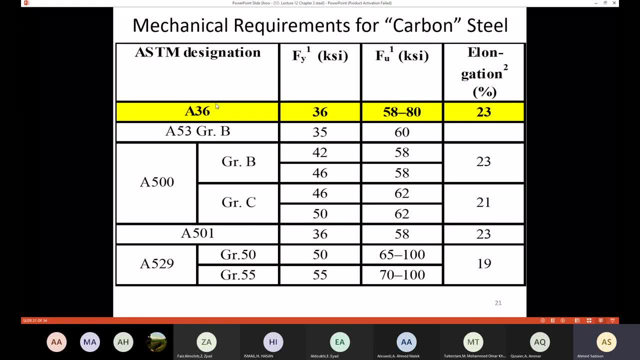 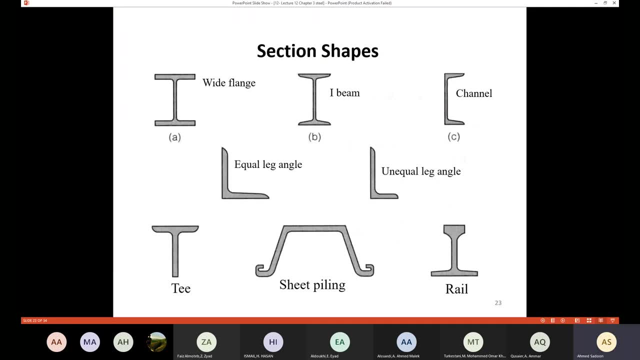 for example, then if you are not sure about who you are going to buy with, then you need to test the, the. you need to test the, the sample of the steel, to make sure that the values is going to meet the requirement. also, we have different section shapes. we have i beam, we have channel, we have wide flange, we have 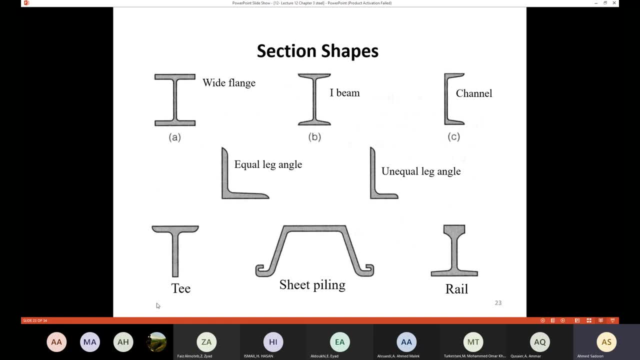 equal leg angle. we have an equal leg angle, we have t, we have sheet piling, we have rail. so also you need to specify the uh, the section, which is section type of the steel, and then you need to specify the type of section that you want. of course, this one is the cross section, okay, so 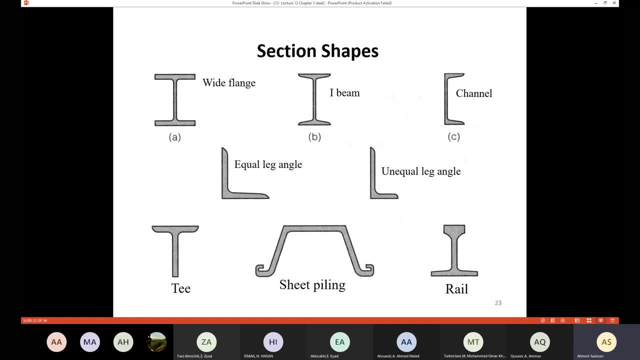 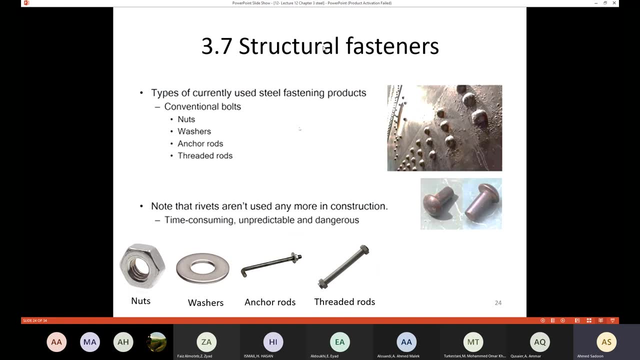 section available through which you can choose whatever you want. also, we have the structural fasteners. we use the structural fasteners in order to connect two parts of the steel. okay, so this one like a connections, and we have the nuts here we picture for the nuts. we have washers. 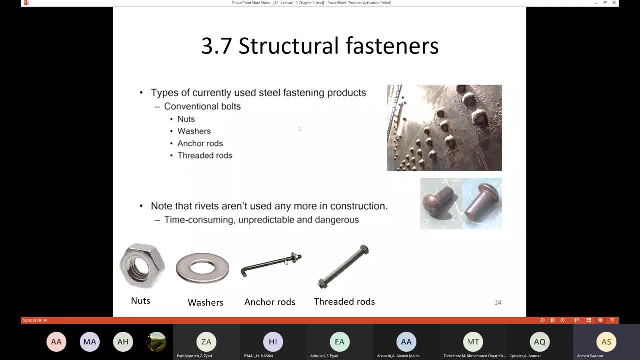 we have anchor rods- this one here, this one is going to be fixed on the ground. we have the threaded rods- this one here, this one also- are going to to connect two pieces of steel. and also we have the rivets. the rivets look like that, very old-fashioned nowadays. 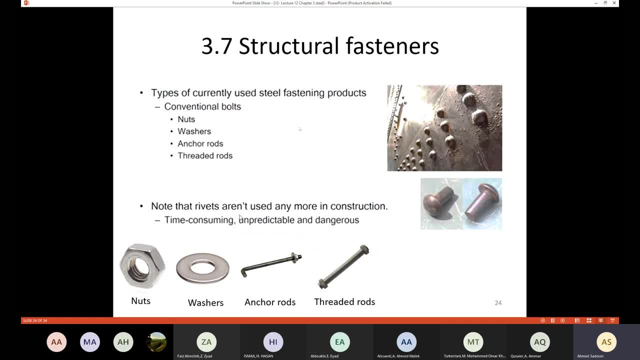 it's rare to use the rivets because it's time consuming. the behavior is unpredictable and it's dangerous. many workers get injured because of the rivets. this one like that, okay. so also we use the steel as fasteners, nuts washers, anchor rods, threaded rods and rivets. 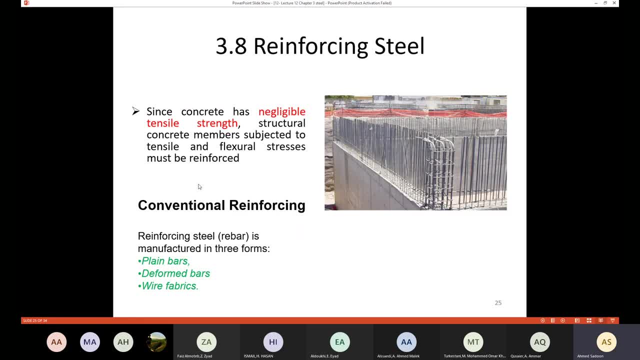 also, we use the steel for reinforcing. we know that the concrete is weak in tension. when we are going to design the concrete, we are going to ignore the tensile strings of the concrete because it's very small and we need to put steel so that the steel is going to take. 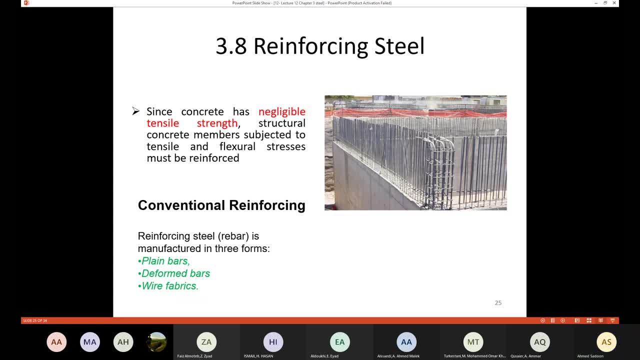 the tensile stresses okay. so if you have a structural concrete member subjected to tensile and fractional stresses, we should reinforce the concrete with steel steel rebars. so the reinforcing steel or the rebar, is manufactured in three forms: we have the plain bars, we have the deformed parts and we have the wire fabrics. so let's talk about each and every. 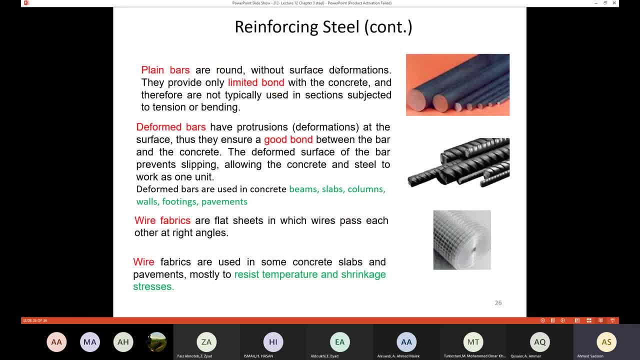 one of them. we have the plain bars. usually they are going to be round like this one here, without service deformation, which means that the service is smooth, like you can see here. so we have a problem with the smooth service because the smooth service, the, the bond between the concrete and the steel, is going. 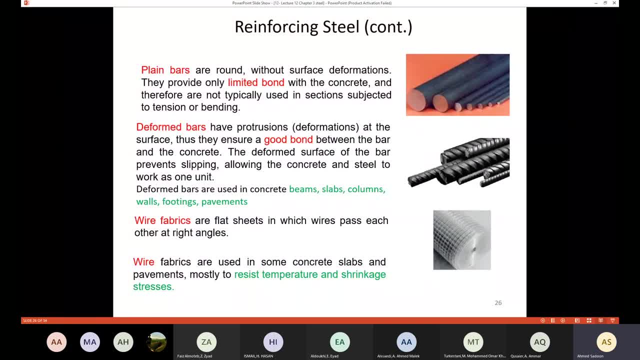 to be limited. they are not going to provide me good bond between them and therefore they are not typically used in section subjected to tension or bending. so we are not going to use this one if i'm going to have tension or bending, because the bond is going to be weak between the concrete. 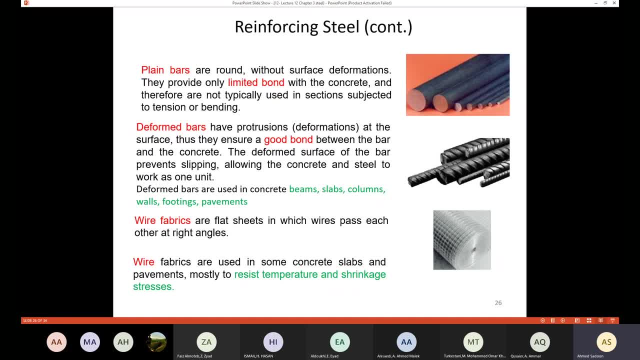 and the steel and the bond between them is very important so that they are going to act like one element. the other one, the deformed bars like this one here. they have protrusions or deformation. we have this one here on the surface. they are going to provide good bond between the bar and 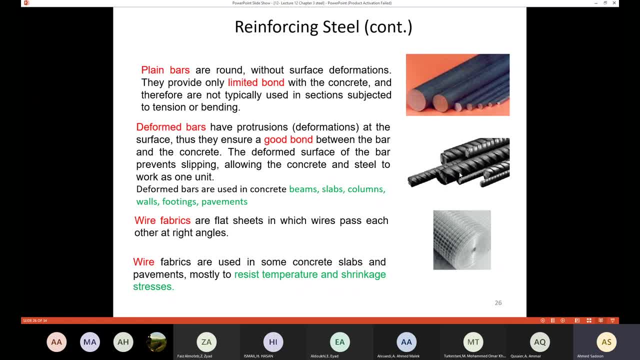 the concrete because of this deformation here. that is going to provide good bond between the concrete and the steel so that they are going to act like one element between the rebar and the concrete. so the form service of the bar prevent slipping, so the steel bar is not going to be slipped and that allowing the concrete and the steel to work as one unit. 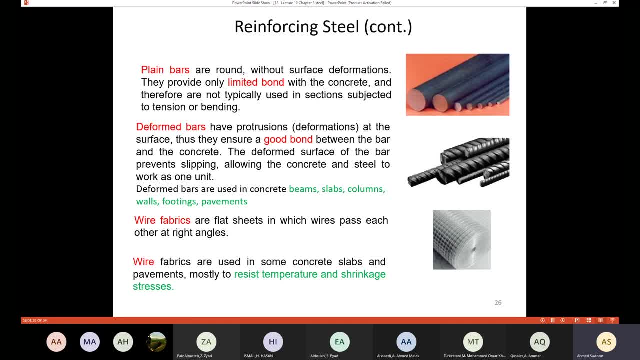 like i just mentioned, they are going to work like a one unit because the bond between them is good. but if you, if the service is smooth, like the blend bars, then the steel is going to slip from the the concrete, okay. so, uh, it's good to use deform bars nowadays. uh, we use the deform bars more than the plane. 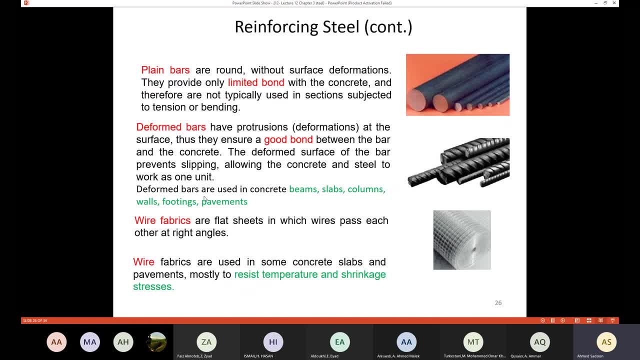 the plane bars. so the deform bars are used in concrete beams, slabs, columns, walls, footings and pavements. in all these applications we use the deform bars. also we have the wire fabrics. look like that, the wire fabrics. they are flat sheets in which wires pass each other at right angle. 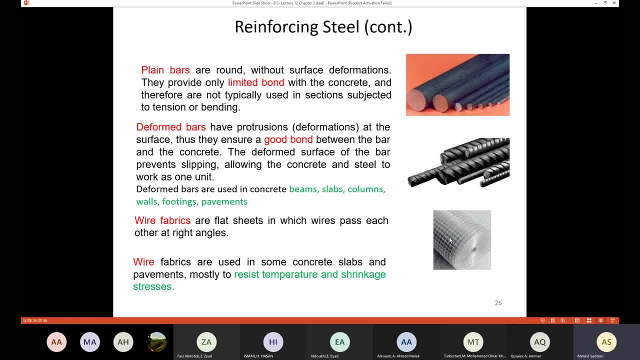 so this one in x and in y, the angle between them is 90 degree. so where we use the wire fabrics, we use the wire fabrics in concrete slab and pavement, mostly to resist temperature and shrinkage stresses. so this one is not, is not going to be used in order to uh. 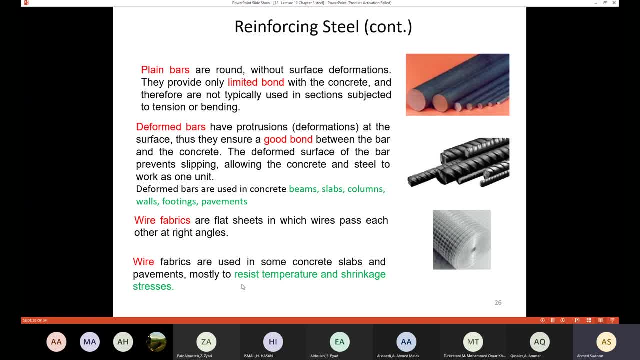 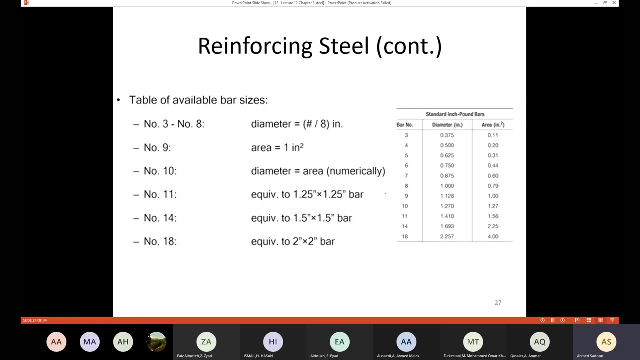 take care of the tension or the bending, this one mostly for resisting temperature, because the temperature might rise or might fall and that is going to cause a problem. so mainly we use the wire fabrics in order to resist temperature and shrinkage stresses. also, we need to know the available bar sizes, those reinforcing steel, they come into bar sizes. we. 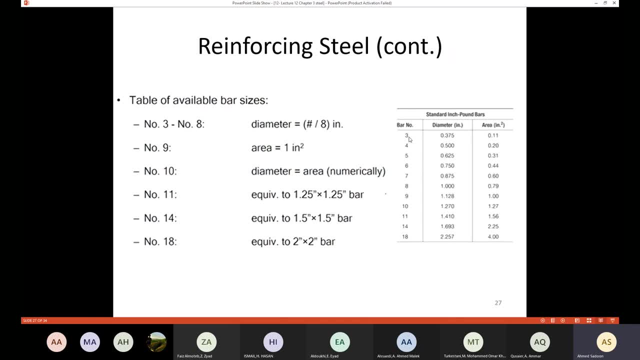 have different bar sizes. so here we have bar number three, four, five, six, seven, eight, nine, ten, eleven, fourteen and eighteen. we have uh different uh bar sizes. okay, for example here, bar number three: it has a diameter of 0.345 inch and the area is 0.1. so each and every bar number it has its own diameter and its own area. 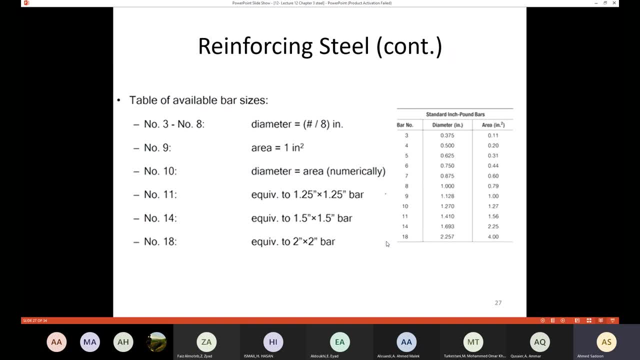 and we have some properties uh regarding the uh bar sizes. so from number three to number eight, here, from three to eight, you can determine the diameter uh if you know the number of the bar size of the steel bar over the number eight. So, for example, in bar number four. 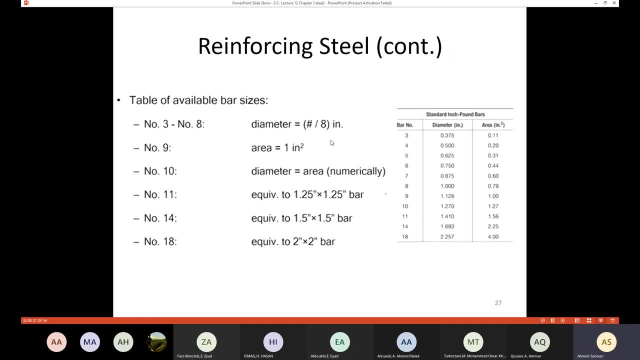 if I wanna know the diameter, I'm going to say that the number is four, I'm going to divide it by eight, and then the diameter should be 0.5.. So, from number three to number eight, I can easily know the diameter using this formula. 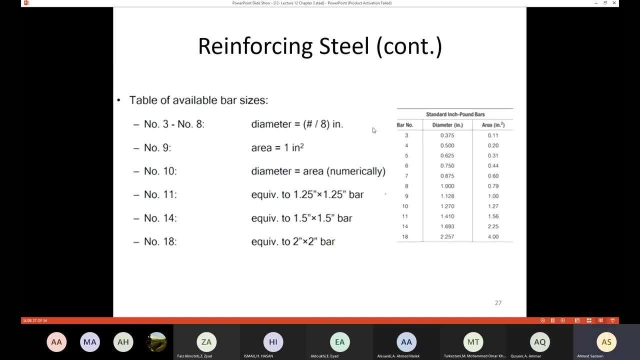 And regarding the bar number nine: here in bar number nine the area is one, It's just special properties regarding the bars numbers. So this one is special number, The area is one in bar number nine. In bar number 10, the value of the diameter. 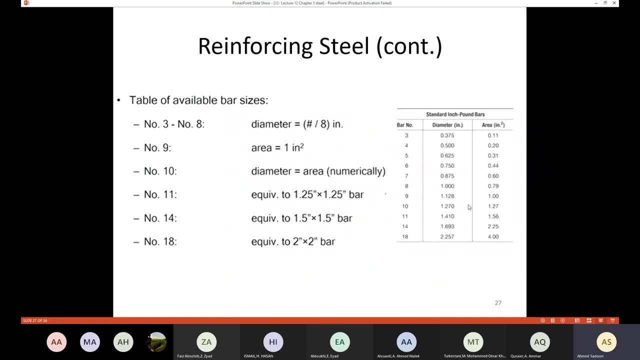 is the same as the value of the area. of course, numerically Okay, because the area and the diameter they represent a different parameter, But here, as a property, the value of the diameter numerically is the same as the value of the area. 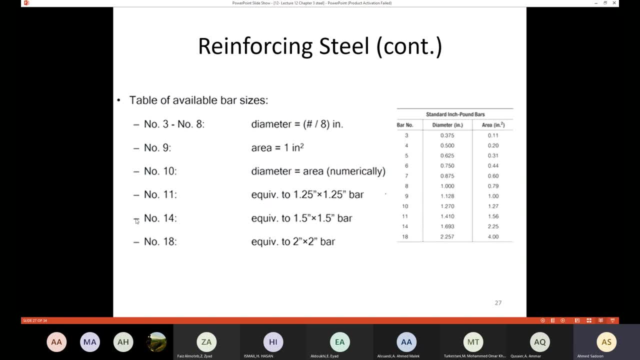 regarding bar number 10.. And also in bar number 11,, this one here, the area here is equivalent to a bar square bar of 1.25 times 1.25.. So just like you have a bar with square cross section 1.25 by 1.25, so if you multiply this value by that value, it's going to. 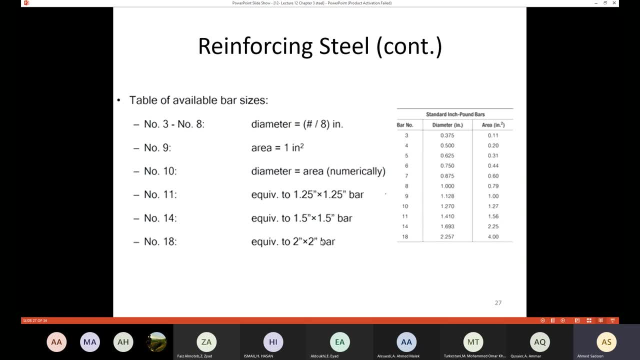 give you this number here: 1.56. also, regarding steel bar, number 14, the area is equivalent to square cross section of 1.5 times 1.5. similarly, in number 19, the area is equivalent to square cross section of 2 times 2. so 2 times 2 is going to give me 4. okay, this is just a special properties. 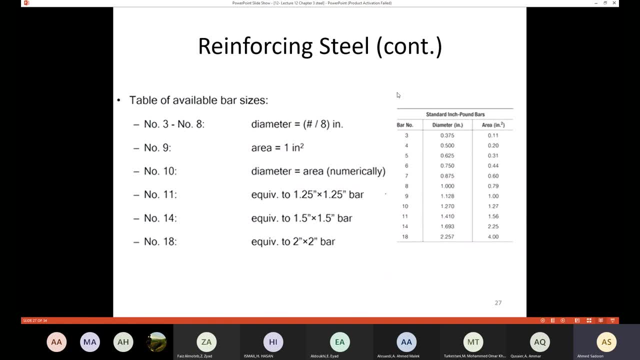 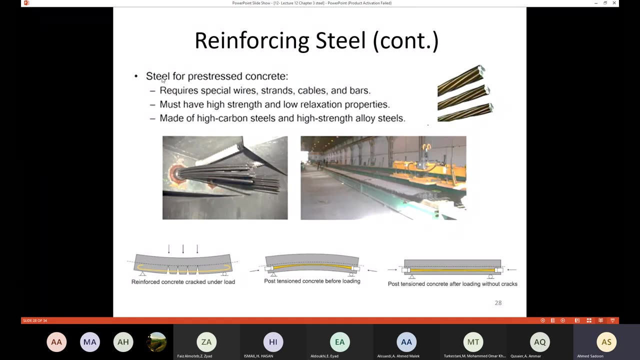 it's very important to understand them. okay, this is going to help you in order to be familiar with the bar sizes. also, we have the pre-stressed concrete. we use steel in pre-stressed concrete, the idea of of the pre-stressed concrete. we know that if you have a beam, for example, like this one, 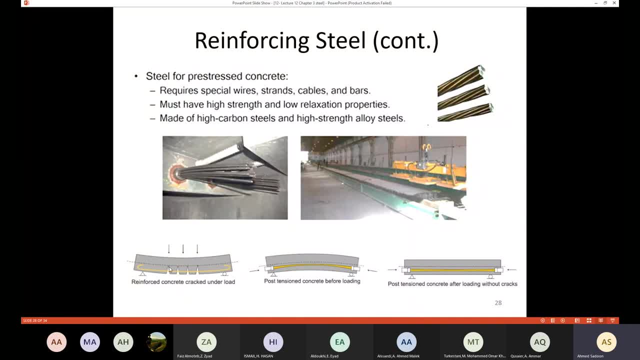 if i'm going to apply a lot, then the lower part is going to be subjected to tension, like we have seen in the lab. okay, regarding the flexural strength, we have done that test. so, uh, because this part here is going to be weak part, because the concrete is weak in tension, then we 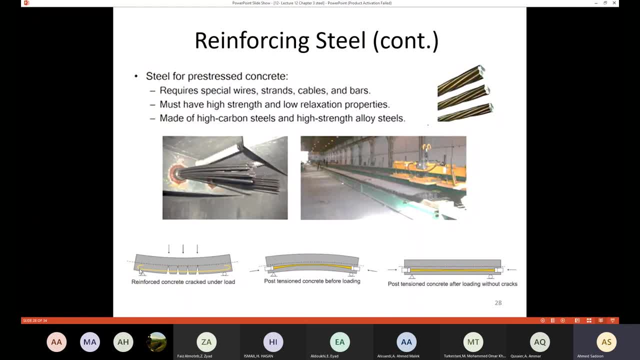 need to put the uh steel reinforcement here so that the steel here is going to take care of the tension. it's a pre-stressed concrete, special type of the concrete. in that one we are going to put cables or wires made from the steel. we are going to place it here, down there. 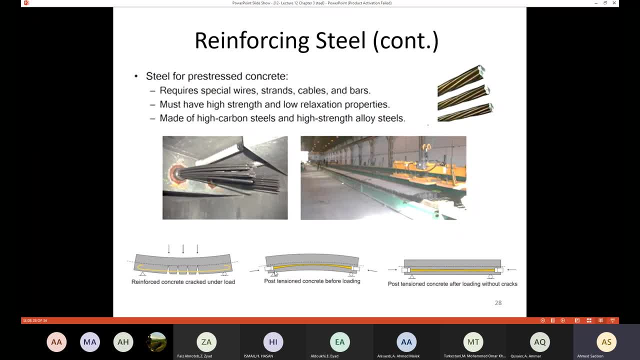 then we are going to apply a force. okay, then we are going to close those gaps here. at the end we are going to apply a force, okay, and then we are going to close those gaps here. if you are going to do that, it's just like you apply a compression at the bottom here. so if you are, 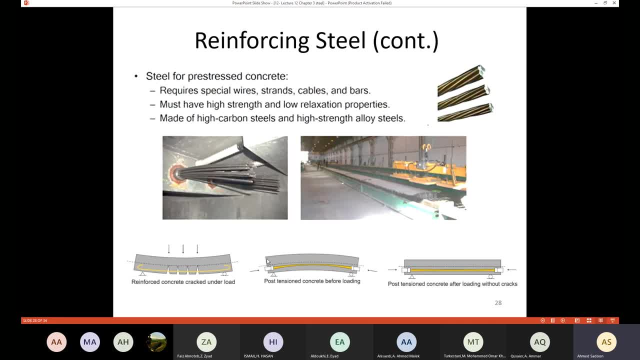 going to apply compression at the bottom, then the beam is going to curve like that, which you mean that here i have compression, i don't have tension anymore. then when i'm going to apply the load again, then the i have already turned a compression here. then when you are going to 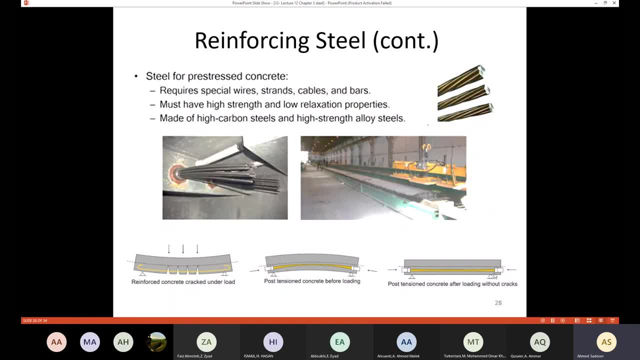 apply tension. the compression is going to balance the tension so that at the end, i'm not going to have any- uh, i'm not going to have any tensile stresses at the bottom. this is the idea of the pre-stress concrete, or the- sometimes we call this the post tension concrete. 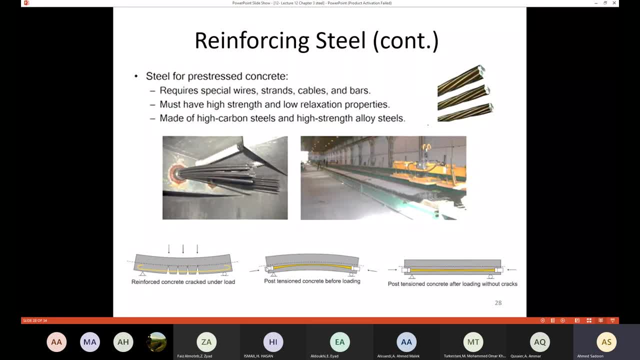 in order to do this process- here we represent the end of the beam- we need special wires, strands, cables and bars look like that. so those those types of the uh special wire, strands, cables and the bar must have high strength and low relaxation properties. okay, and they should be. 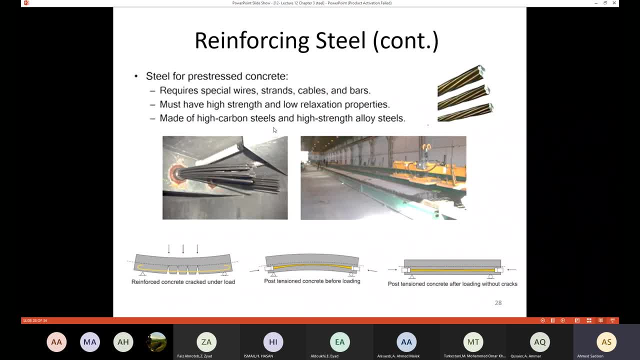 made of high carbon steels and high strings alloy steel, so this one should be made of high carbon steel. so here we don't want ductility, we want strength. so we are going to use high carbon steels and also we are going to use uh uh allowing steel in order to enhance the strings more and more. 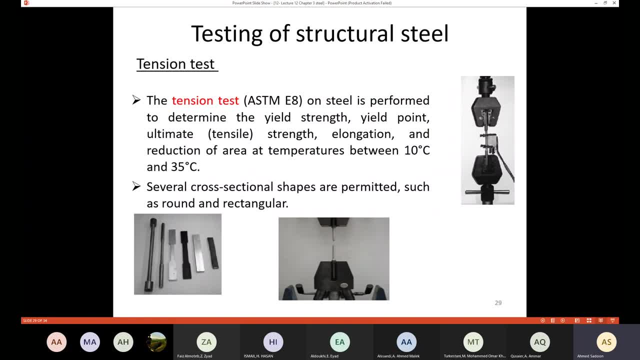 finally, we need to understand the test that should be performed on the structural steel. of course, the most uh important one is the tension test. also, we have that in the lab, the tension test. so the tension test according to astim e8 should be done according to that uh standard. uh, the the tension is still uh. the tension test on steel. 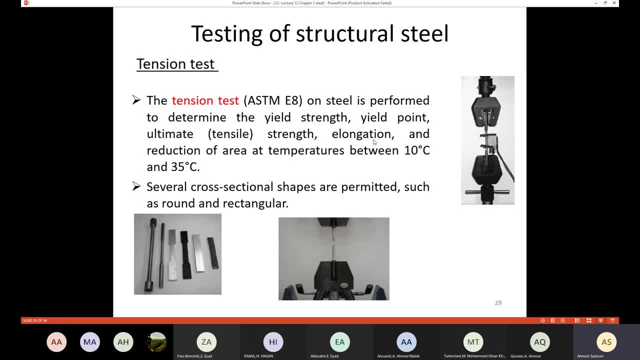 is performed to determine the yield strength, the yield point, the ultimate tensile strength elongation and the reduction of the area at temperatures between 10°C and 35°C. So the purpose of the tension test, in order to know all of these properties. 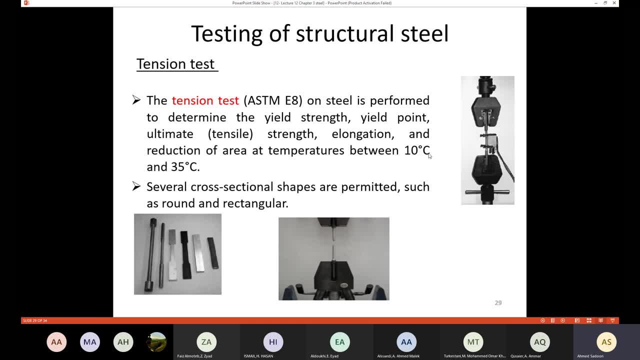 the yield strength, the yield point, the ultimate strength, the elongation and the reduction of the area at the temperatures between 10°C and 35°C. So the test should be done between those temperatures. We have several cross-sections. 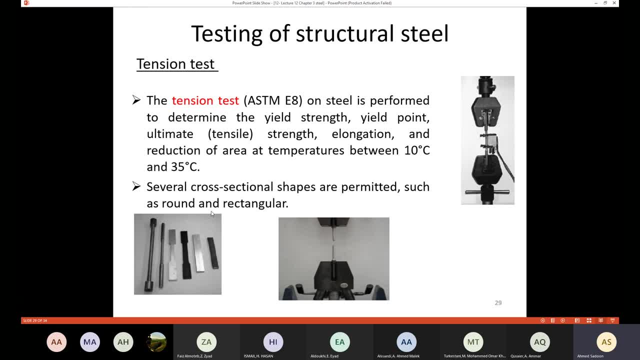 Shapes are permitted, such as round and rectangular, So you could use many types of the specimen. Mainly the most used one is the round cross-section. Then we need to place the steel bar into this machine, the tension machine, And then 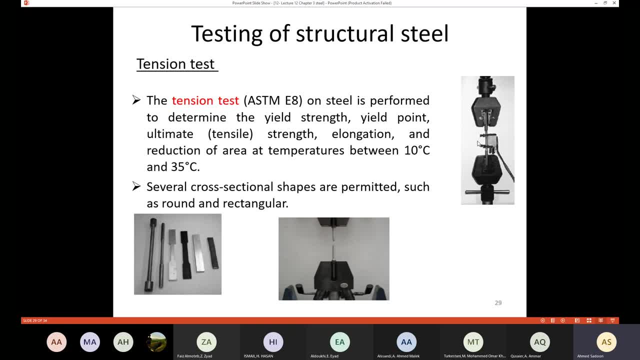 we need to attach a recorder in order to determine the elongation And also we need to have something in order to record the load. We need to have cell load in order to record the load And also we need to have maybe LVDT in order to determine the elongation. 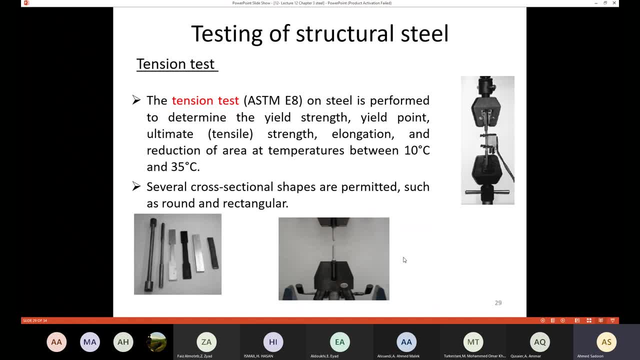 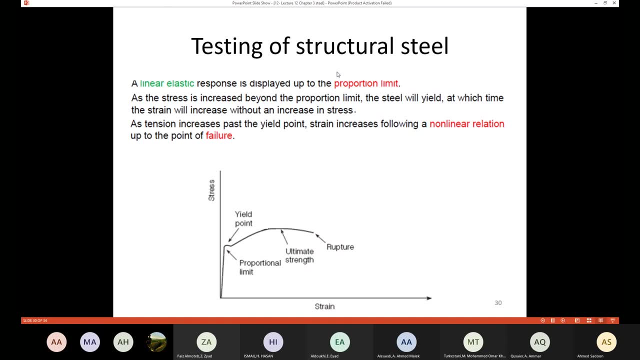 And then all of these values should be recorded so that you can generate the stress-strain diagram. You are going to apply a force up to phase, So after you apply this test, then the stress-strain diagram is going to be generated. 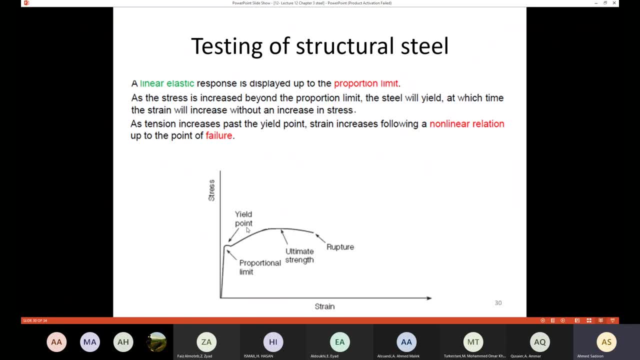 And you are going to know the proportional limit, the yield point, the ultimate strength and the curvature. The linear elastic response is displaced up to the proportional limit. So up to the proportional limit here we are going to have elastic response. Then, as the stress is increased, when we increase the stress beyond the proportional limit, the steel will yield. 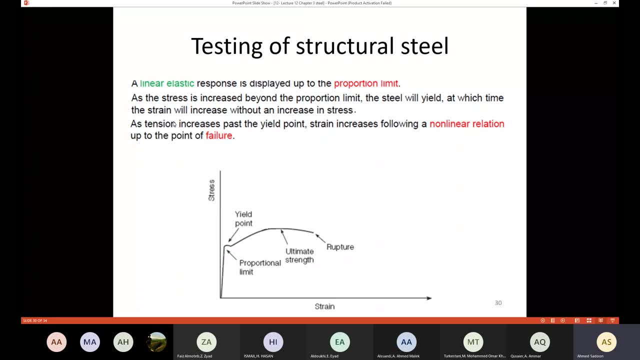 Yielding. it means that the strain will increase without an increase in stress. So here the strain is going to increase without any increase in the stress. We call this level or process, we call this yielding. Then after that, as tension increases, 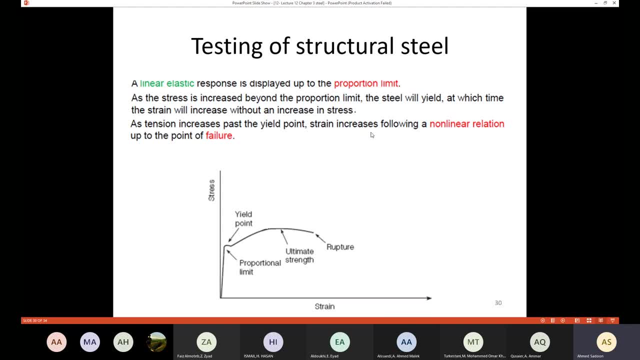 as we pass the yield point, the strain increases, following a non-linear relation up to the point of failure. So after the yield point here the behavior is going to be non-linear, While the behavior before the yield point is going to be a linear behavior in general. 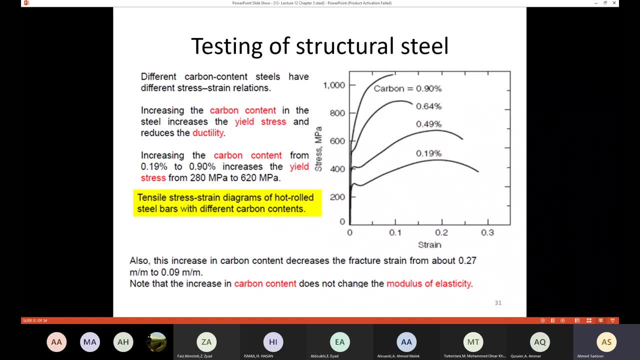 So also we need to understand the effect of the carbon on the stress-strain diagram. So in this graph the tensile stress-strain diagram of hot-rolled steel bars with different carbon contents. So here we have conducted many tests with a different percentage of the carbon. 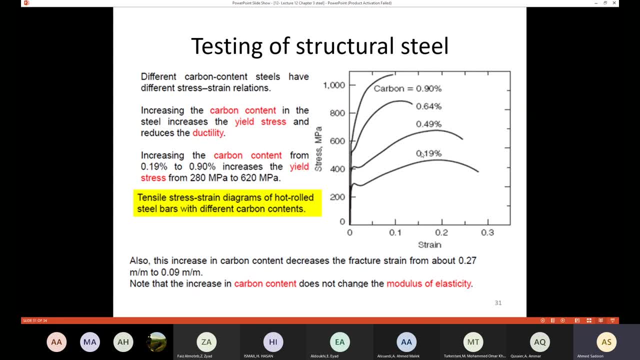 So in the first test here, the percentage of the carbon is 0.19%, Here is 0.49%, And here is 0.64% And finally here is 0.9%. So we need to know this. 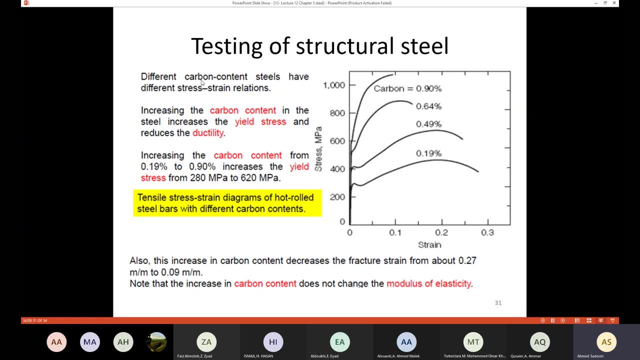 The effect of the carbon percentage. So different carbon content, steel level have different stress-strain diagram relations. The stress-strain diagram is going to be different Then increasing the carbon content if we are going to increase the carbon content in the steel. 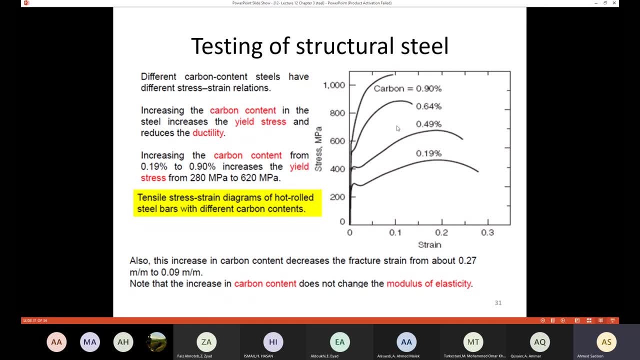 then the yield stress is going to be increased. So here, if I'm going to increase the carbon percent, then the yield stress is going to increase And the ultimate stress, of course, is going to increase as well, But the ductility is going to be reduced. 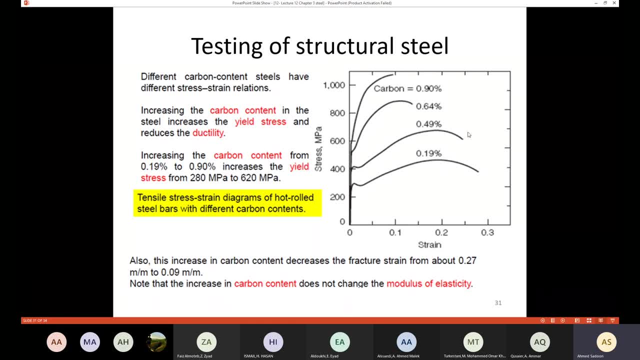 So you increase the percentage of the carbon, But here the ductility decreased, Decreased and decreased. So increasing the carbon content from 0.19, from this value to 0.9%, to that value, then that is going to increase the yield strength from here, for example here: 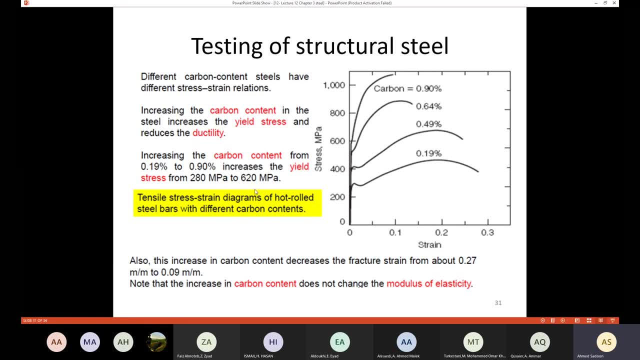 from 2.8 MPa to 6.20 MPa here. So the yield strength is going to move from 2.8 MPa to 6.20 MPa, Okay. Also, this increase in the carbon content decreases the fracture strain from about 0.27 here. 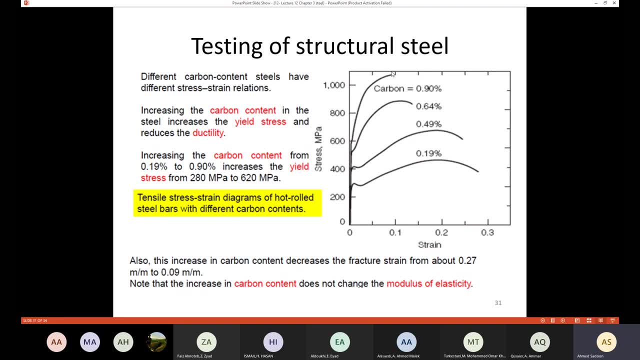 0.27, to 0.9%- 0.09. here The fracture strain is going to decrease. But you need to understand this: Even though we have all of these changes, the value of the modulus elasticity is going to be the same. 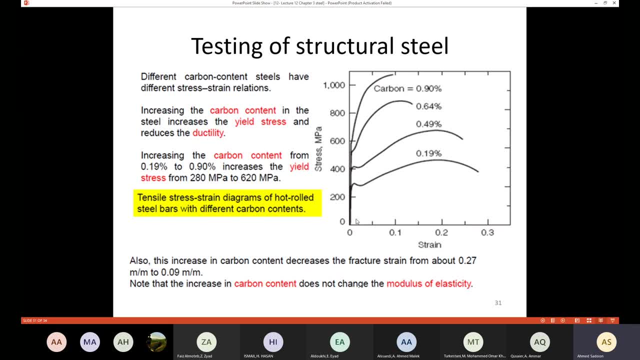 So here, if you measure the slope here, which is the modulus of elasticity, it's going to be the same for the different type of the carbon. You need to remember this Also. we have the torsion test Also. we have done that test here. 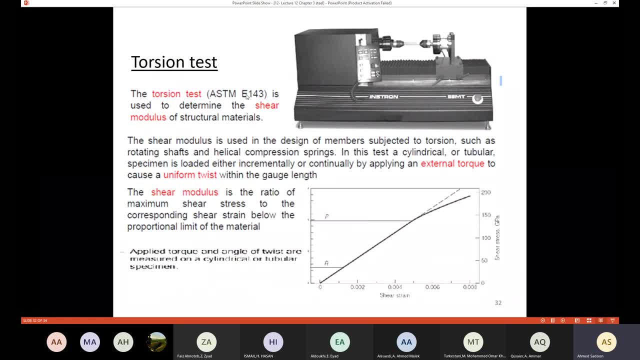 The torsion test should be conducted according to ASTEM E143. And this one is used to determine the shear modulus of structural element. We know that the shear modulus is important, especially in the member subjected to torsion, such as rotating shafts in the cars and into automobiles, and so on. 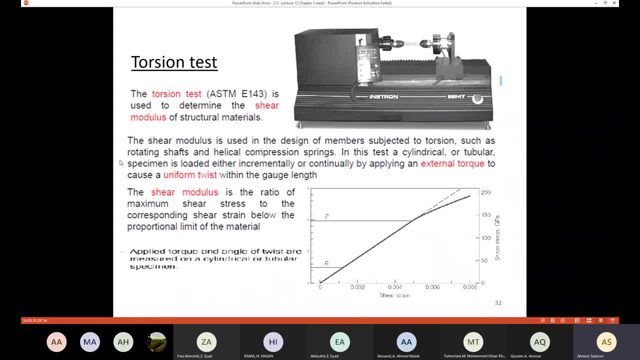 And in this test a cylindrical or tubular specimen is loaded either in critical or continually by applying external torque. So we are going to place the specimen here And we are going to apply external torque in order to cause uniform twist within the gauge link. 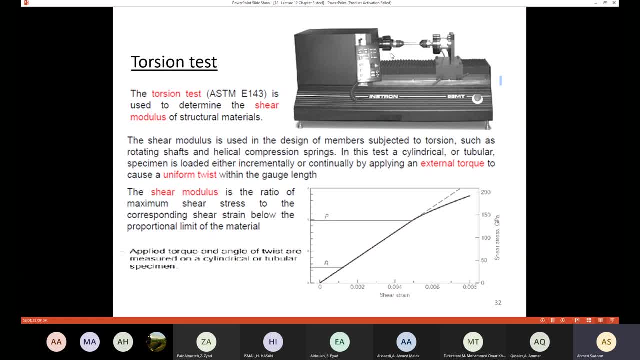 Within this link we are going to cause uniform twist And you are going to apply the torque And also you are going to get angle of twist. So you need to measure the torque and the angle of twist so that you can generate the torque. 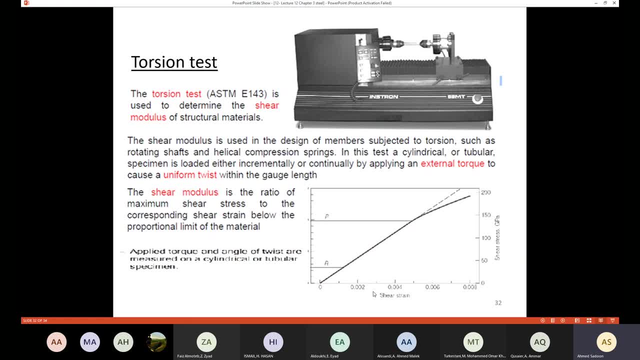 To generate the shear strain And then, if you come up or if you manage to generate the stress, the shear stress and the shear strain, then you will be able to determine the shear modulus, which is the ratio of the maximum shear stress to the corresponding shear strain below the proportional limit of the material. 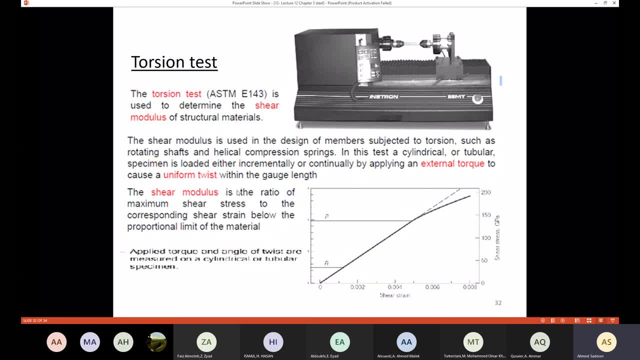 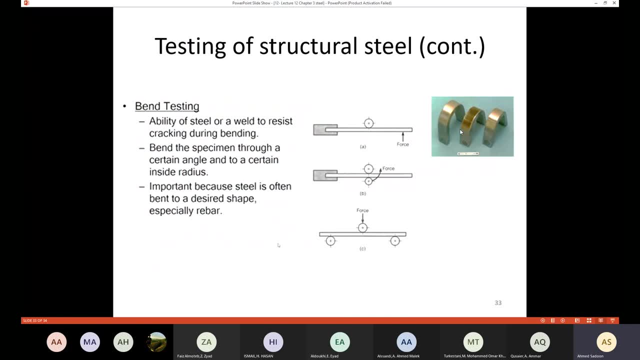 So if you measure the slope of that line then you are going to determine the shear modulus. Finally, we have the bend testing. The bend testing is important because usually we are going to bend the steel, So also we need to know the ability of the steel to resist cracking during bending. 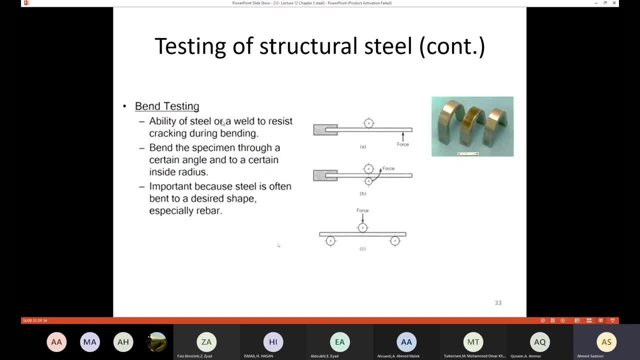 So the bend testing is the ability of the steel or a weld to resist cracking during bending. We are going to bend the specimen through a certain angle and to a certain inside radius. So here we are going to put those rollers, here We are going to apply a force so that we know that how much we can bend the steel.